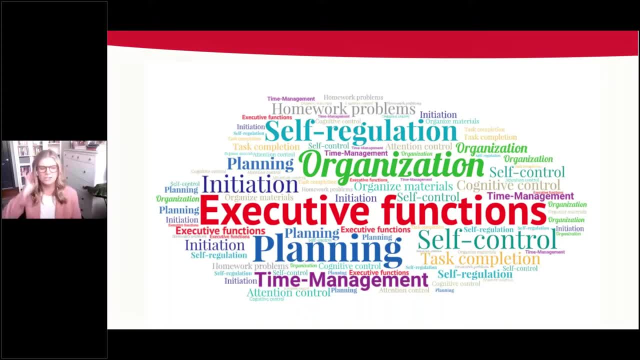 an executive functioning disorder. executive function treatments or interventions, And what executive functions are, are really? it's an umbrella term that refers to cognitive processes that are necessary for completing goals, Or they're actually more of a goal directed behavior, And so that includes things like 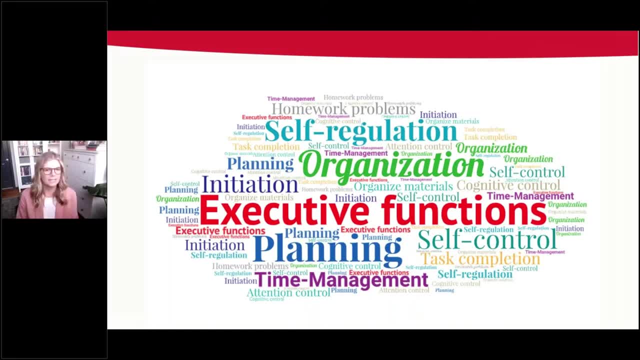 intimidating certain behaviors in order to do other behaviors, planning ahead, self-regulating not only behavior but emotions and actions and tasks, completing tasks, planning ahead and managing one's time. So these executive function skills, you can kind of sometimes I call them the conductor of the orchestra. 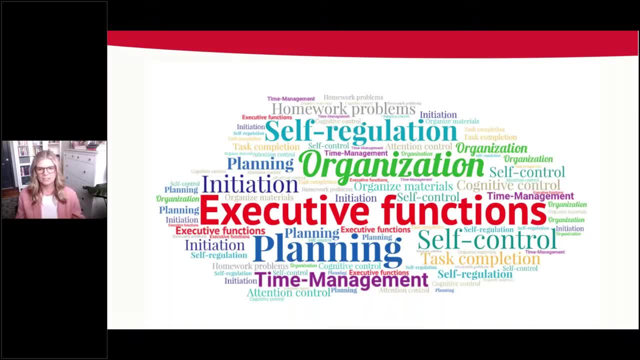 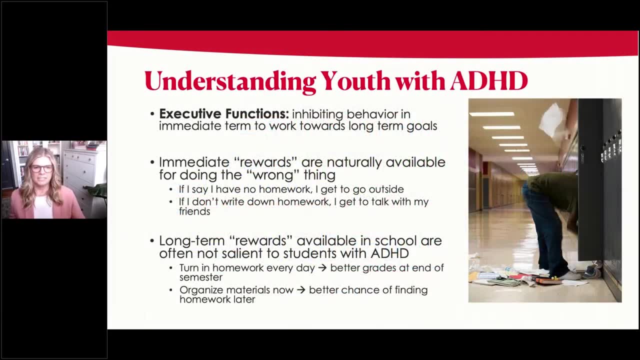 because they're really responsible for the sort of more complex skills that start to develop in early and are important throughout development, And so I think it's helpful in understanding what the role is of executive functions for youth with ADHD. So if executive functions are the conductor of the orchestra, they're really responsible. 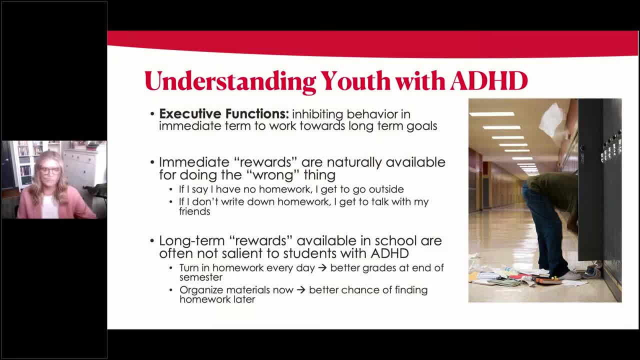 for monitoring and controlling what happens in the moment, the immediate behavior, and how that is working towards or against their long-term goals. So one thing that we often see in the school context and at home when it comes to completing homework with youth with ADHD is that the immediate rewards those that are naturally 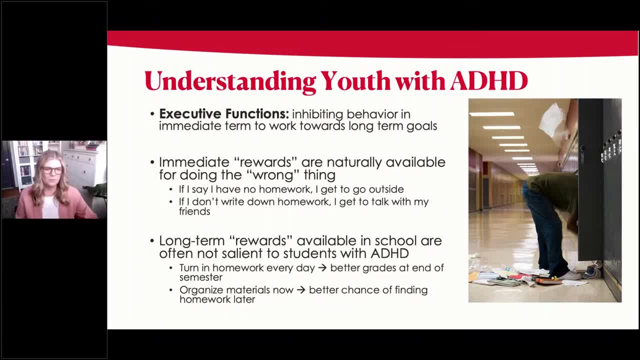 available. those are often rewarded for doing the wrong thing, And what I mean by that is in the moment they might be drawn to doing things with their peers or not completing their work. other distractions: maybe their favorite TV show is about to be on. 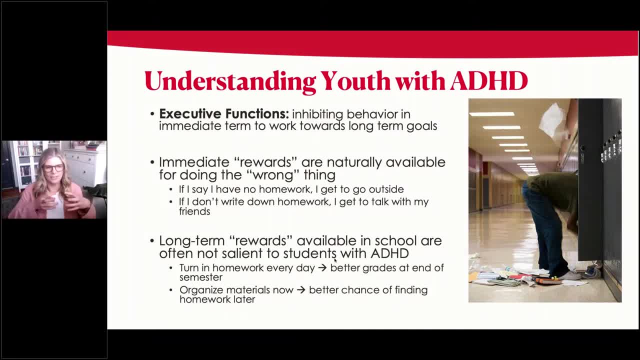 And there's a lot of distractions in the world that are more appealing, that are right in front of them, than the longer-term, more abstract thing, such as my grades at the end of the semester or how I'm going to do on a test. that's not until next week. 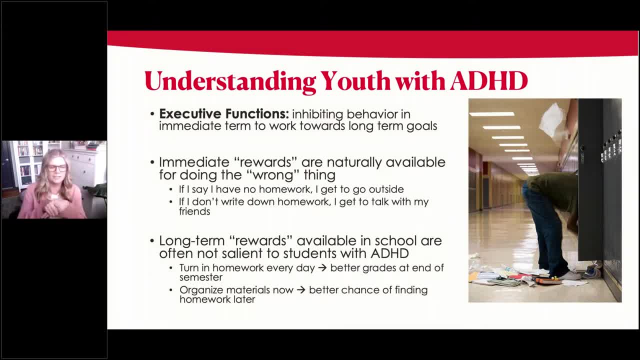 So it can be really difficult to kind of work towards those longer-term goals, especially when there's all these immediate distractions right in front of you. So I put here: you know, if I say I don't have homework right now, then I get to go. 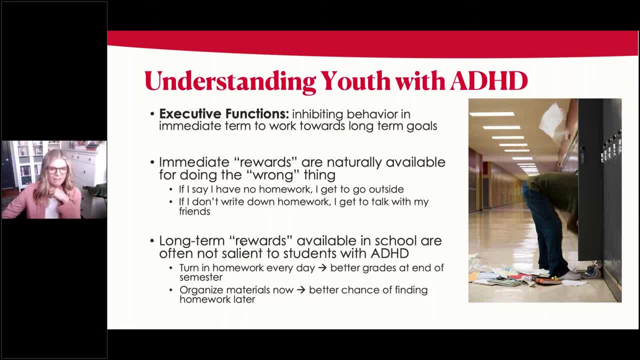 outside, I get more free time. If I don't write down my homework at all, then I get to immediately after the end of the class. instead of taking five minutes to do that, I get five minutes more in the hallway with my friends. 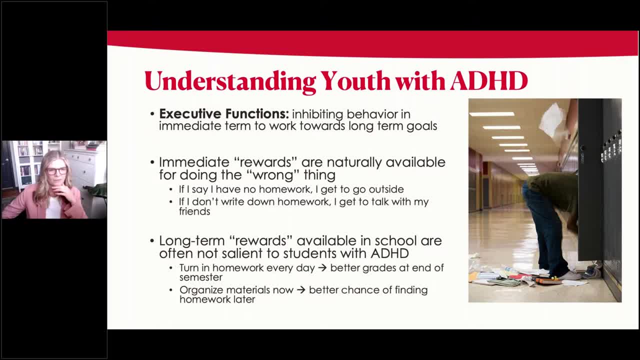 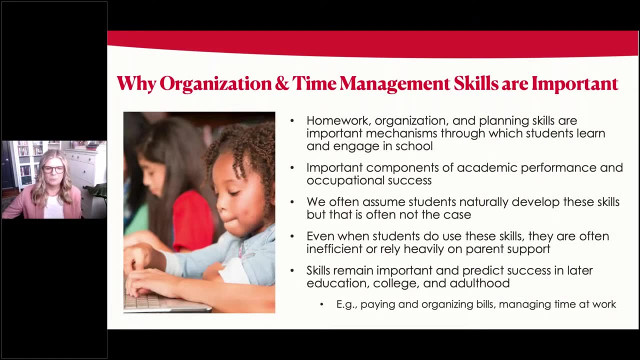 So you can kind of think about how all those immediate distractions are rewarding for doing the wrong thing And it makes those longer-term rewards particularly challenging, especially for youth with ADHD, because they seem more abstract and less tangible. So why organization, time management skills are important? 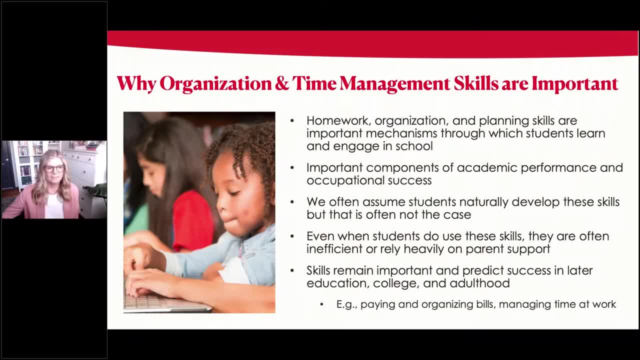 So school Historically focus on teaching material things like math skills, science skills, other languages, English and obviously those academic skills are highly important, but without organization, time management and planning skills they don't allow a student to really engage in what they're learning and achieve their full potential. 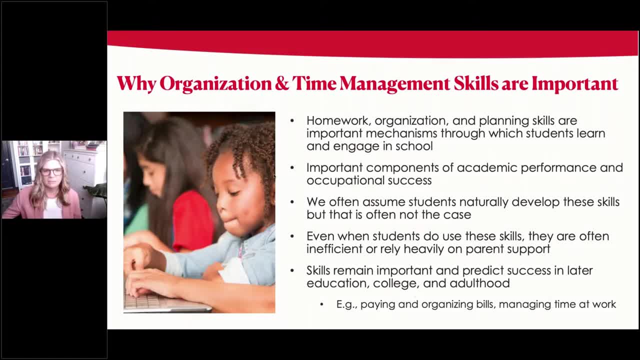 And in our work, we believe that kind of these organization and time management skills are just as important aspects for us to teach. So, Yeah, Yeah, And to be able to teach and encourage students to do as as the material itself and they're. 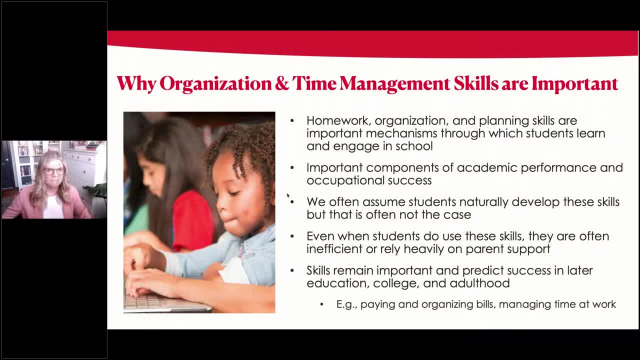 important not just for right now, for students in elementary, middle or high school, but also later in life, as they transition either to college or to occupational settings. It's important to be able to have these organization skills, time management and planning to be. 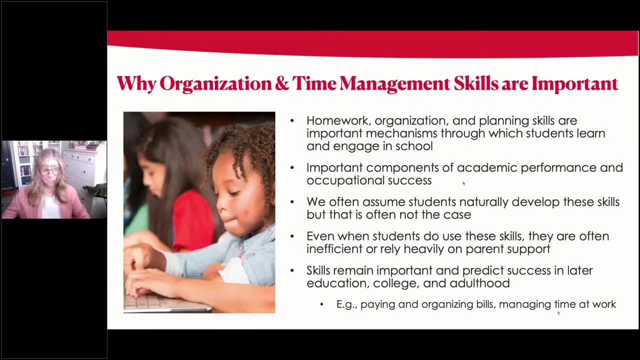 able to adapt well and be successful in other situations too. So we often assume that these skills are they just develop as as one transitions, say, middle school, and that they'll just be there and that they'll know what to do and they'll know how. 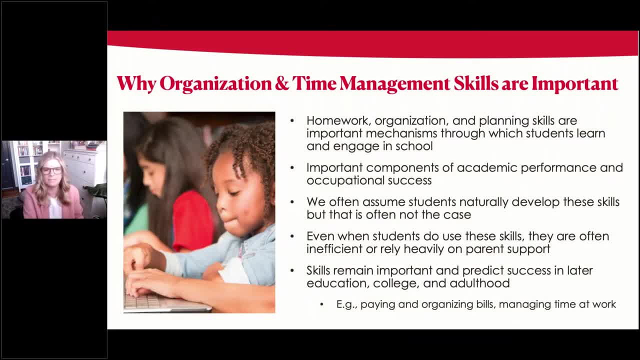 much to record in their planner or their calendar and kind of what it means to be organized, But that's often not the case And it's particularly challenging for individuals with ADHD. coming back to some of those executive functioning difficulties, We see homework organization. 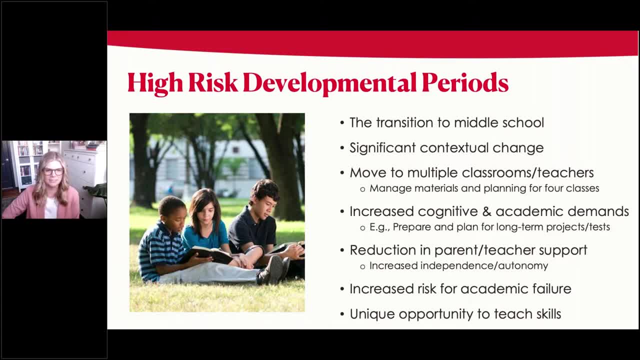 and time management difficulties really start to arise at key points in development. So one really important period of development is the transition from elementary to middle school, And this represents for a lot of kids a big shift going from one teacher to multiple classrooms, multiple teachers, And for parents too that means kind of managing expectations for four or five. 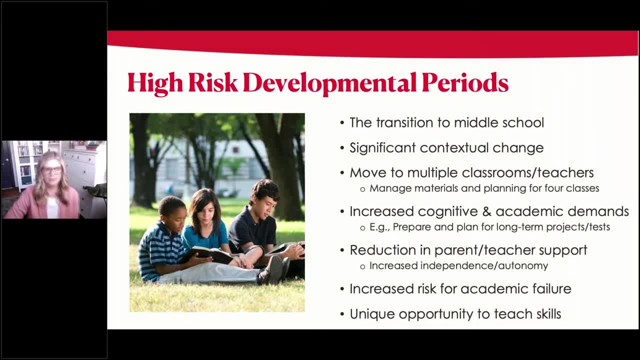 different classes, teachers, some who might use some online platforms for assigning homework, others don't. some write things on the board, some might just say it verbally in the last five minutes of class. All these different kind of methods of their own organization and ways that assignments are given. 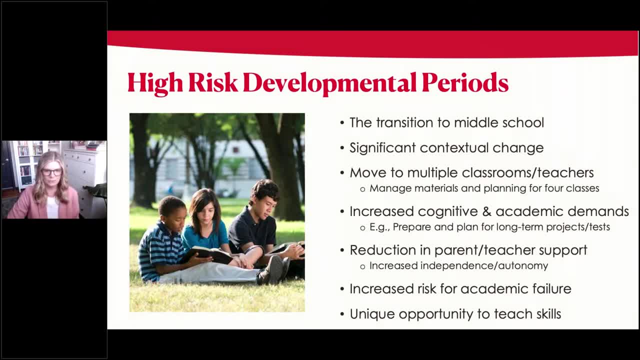 it makes it very challenging for all students really to be able to keep up with. And there's also this at the same time: this kind of reduction in teacher support by having multiple students and instead of, you know, 20 or 30 students in the day that the teacher is responsible for. now they have. 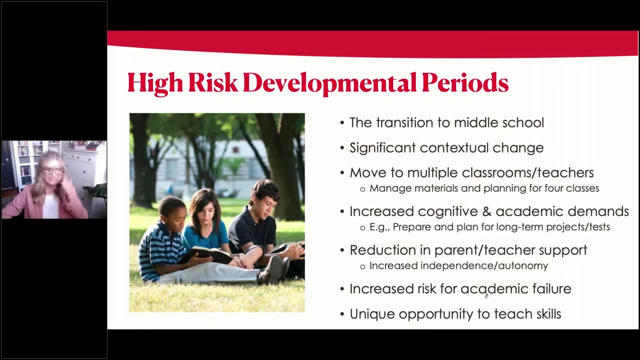 hundreds that are cycling through their classrooms. So there's sort of less teacher contact sometimes in the transition to middle school And it's a really high risk period for students to start falling through the cracks. but it's also on the positive side. it's a unique opportunity to really teach these homework organization skills. 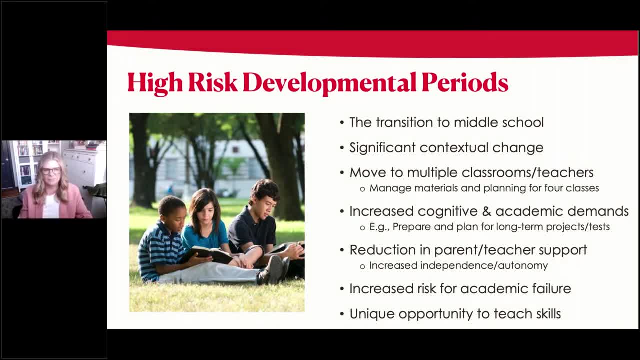 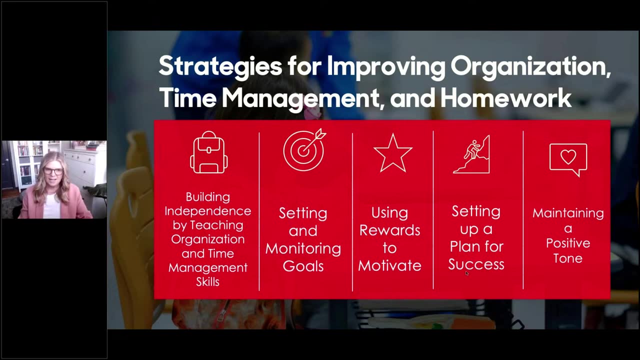 We see an increase in homework demand, and so it's a great time to start working on these skills and in teaching and applying organization, homework and time management strategies. So with that, these are kind of the five areas that I want to talk with you all about today. 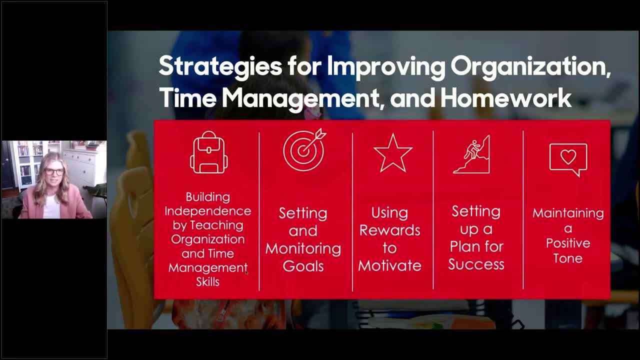 for how to support your student with organization, time management and homework. So I'm going to first talk through some specific strategies for organization, time management and homework skills and ways that those skills to your child or adolescent. But one thing that a lot of research and our interventions hold true to this model is that ADHD. 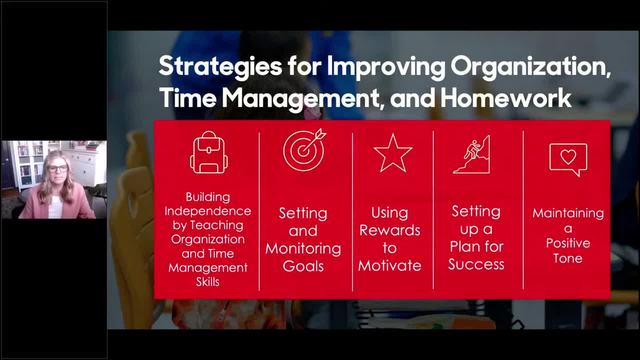 it's not always just a lack of knowing what to do, but it's the sort of the ability to regulate one's behavior and do the right thing In the moment. so you might know that you're supposed to write down homework assignments in your planner. 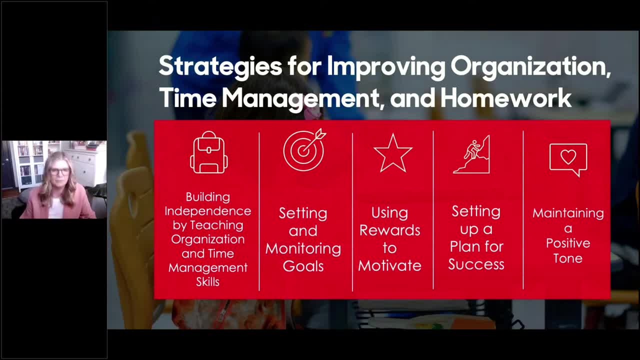 but actually executing and doing that in the moment is what's challenging for you because of some of those inattentive symptoms. So we're going to talk about ways to set and monitor those goals and behaviors around organization, time management, how to use rewards effectively to motivate your child or teen, setting up a plan for success and what that looks like. 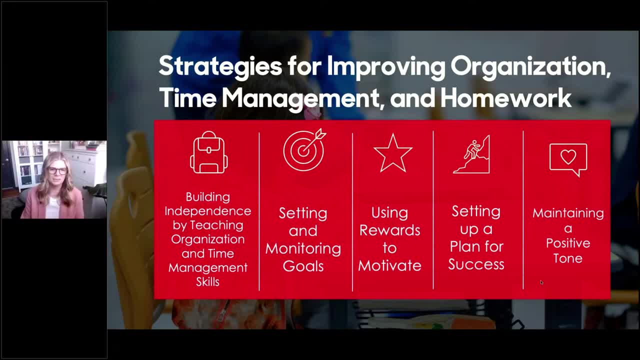 And lastly and most importantly, kind of how to introduce this with a positive tone in a way that's that's going to engage them and feel like an opportunity rather than another task that they have to do. So I think everyone came here today. 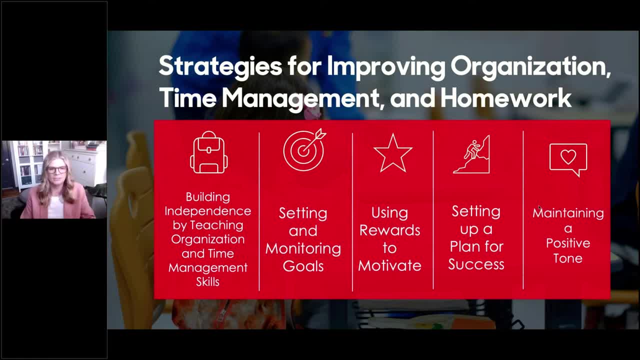 probably thinking about this- first steps, that these last four are really important for making whatever system that you come up with and that you develop as a family or for child students to be successful. So I also want to say that a lot of these interventions and strategies- 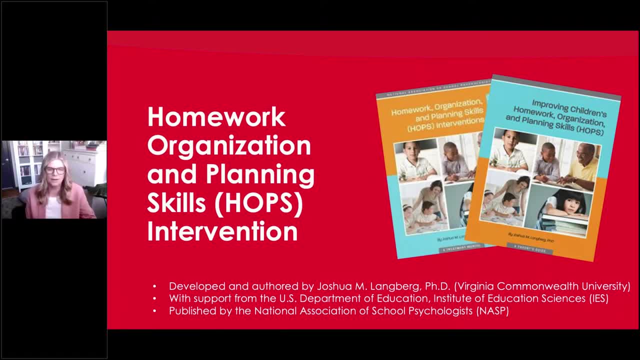 then I'm going to share today actually came from my graduate school mentor. Joshua Langberg wrote a book called homework, organization and planning skills, or hops intervention, And the first book was written for school mental health providers, So people like school counselors, school. 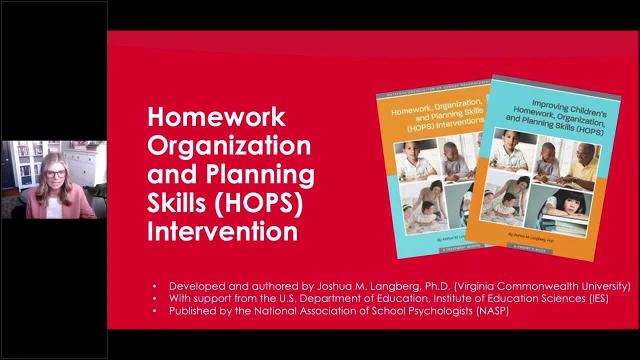 social workers or school psychologists to deliver this program during the school day and in the context of schools. But he's also since published a book specifically for parents that gets into specific strategies for monitoring. So I'm going to share with you a little bit about the process of monitoring homework and organization and time management. 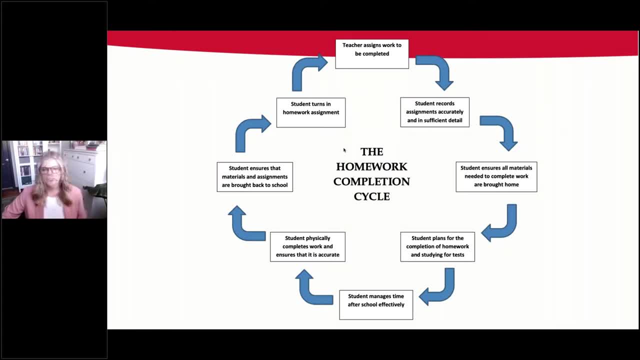 This homework completion cycle is something that we we talk about in the hops intervention, but it's it's important when working with a student with ADHD to think about kind of where is the most impairment, kind of where is the most struggle when it comes to homework. 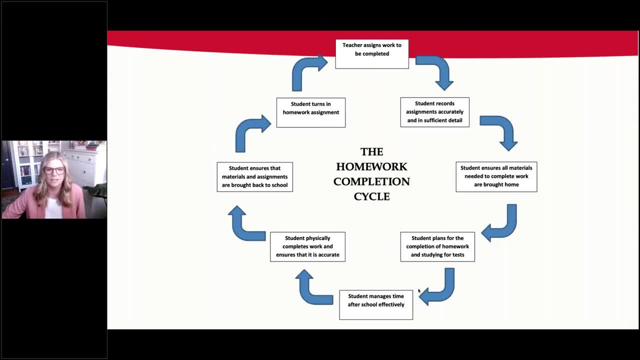 This homework completion cycle kind of shows you each step of the process. There's a lot of areas and entry points for potential difficulties. That one's It's a lot of what I'm going to talk about today, So I'm going to start off with what you're going to need to do to get to your master's degree. 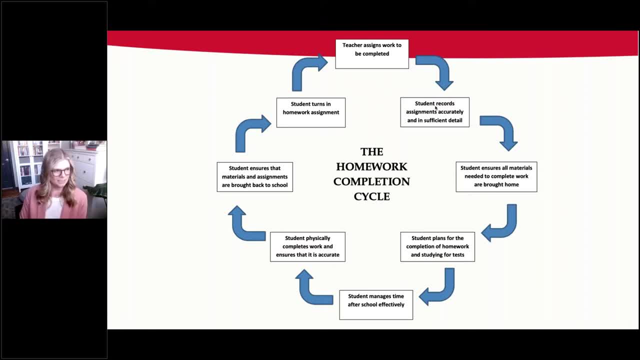 So the master's degree is your master's degree in social work. So you're going to have to complete the master's degree in social work. So the master's degree is going to be for people with ADHD symptoms who get in the way. So it starts with the teacher. 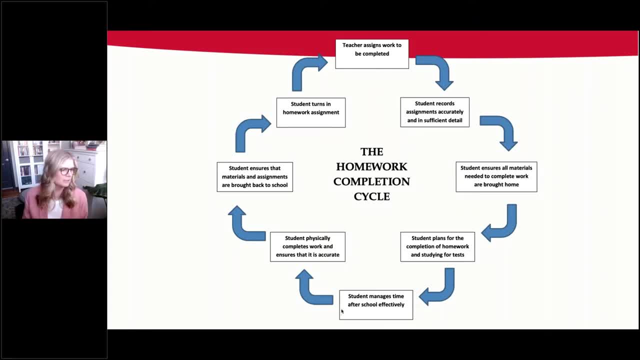 assigning work to be completed. The student then has to actually record the assignment after accurately than enough details. So you know what to do. bring those materials home. plan ahead for tests before, before they happen. manage their time When they're actually. 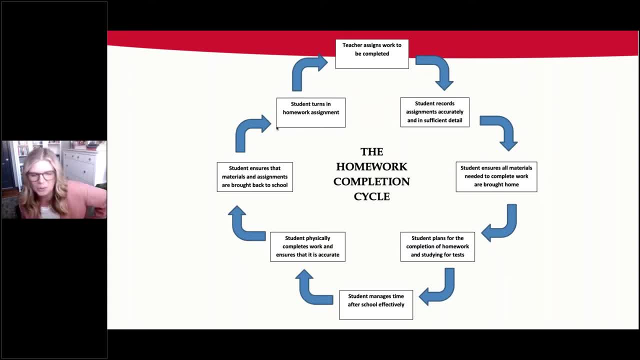 We have families that will help their student with their homework or work on ensuring that their homework is completed the night before, And then something happens the evening before and this homework gets misplaced or it's just forgotten to be turned in. So there's a lot of places where you could initially work on it. 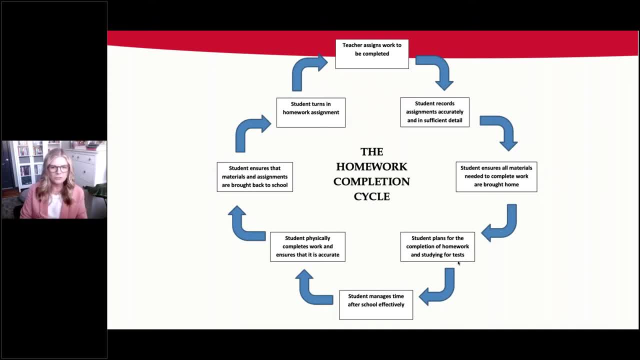 Sometimes we show this as a map to families. You know, there's maybe multiple areas with your child or adolescent that you might want to target. Let's start with one area that seems to be the most problematic and then kind of move into these other areas. 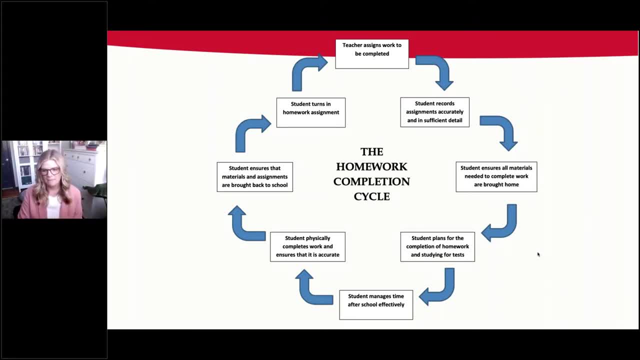 So I'm going to talk about, specifically organization, time management and planning strategies today. There's a lot of other strategies that we'll go into too, but these are helpful in just thinking through where should we start and where should we go from there. 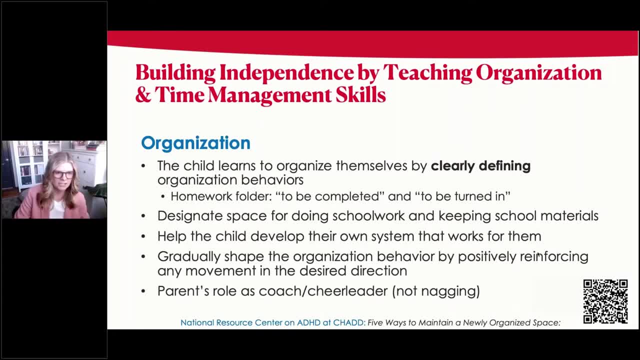 So starting with just organization, So this is one kind of module or strategy to try. So with organization, what we've Find is helpful is that we first focus on clearly defining what it means to be organized And, given that this isn't something that's often focused on it by schools, that means kind of taking time to define what our expectations are around being organized. 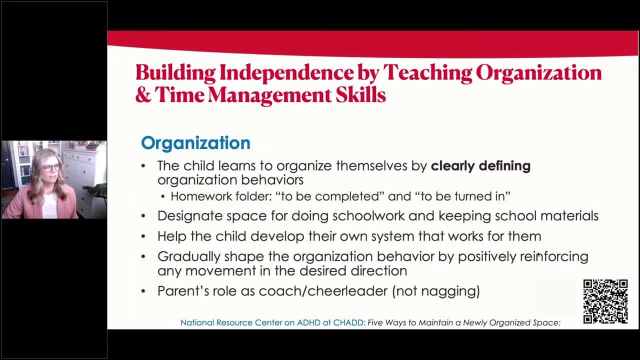 And sometimes, if you ask, what do you want to see, And they say, well, I just want them to be better organized, The child and the parent might come up with 10 different definitions of what that means. And so by, By sitting down and 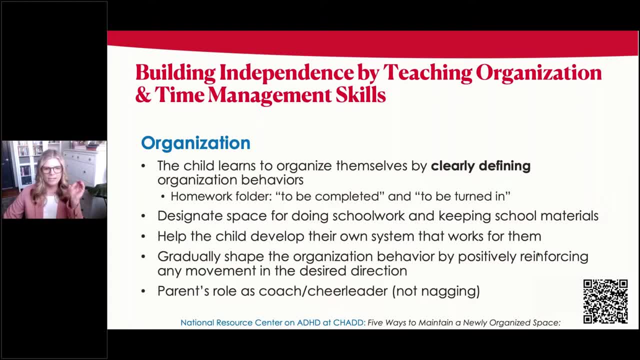 Writing Out these expectations of what it means to be organized very specifically. it really is. the goal here is so that way both parties, or all parties, kind of understand what the expectations are, what it means to be organized and what that, what that actually looks like. 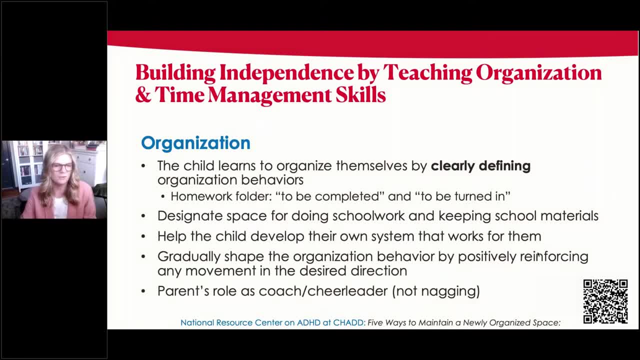 So something that you can is sort of observable and measurable. So in In our interventions this focuses on designating a, a space for doing schoolwork and for keeping school materials, And And parents can help the child sort of develop a system that works for them, whether that is setting up a desk space at home or kind of creating an organization checklist for what goes in the book bag the night before going back to school or kind of what's expected to be in the book bag and what's not to be in the book bag when they make at home. 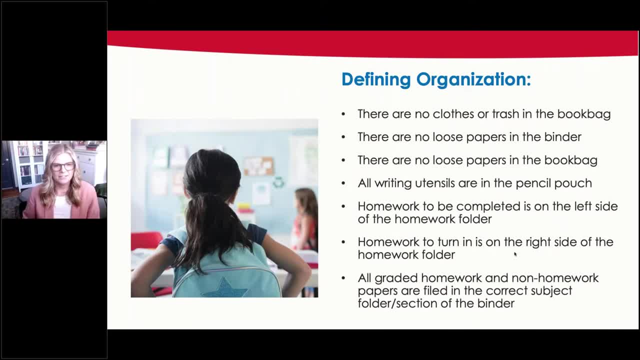 And so we talk about defining organization, and here are just some different examples of definitions of being organized that we've used. there's been other examples of organizations that we've used with families that we've worked with, So it might be things like no clothes or trash in your book bag. 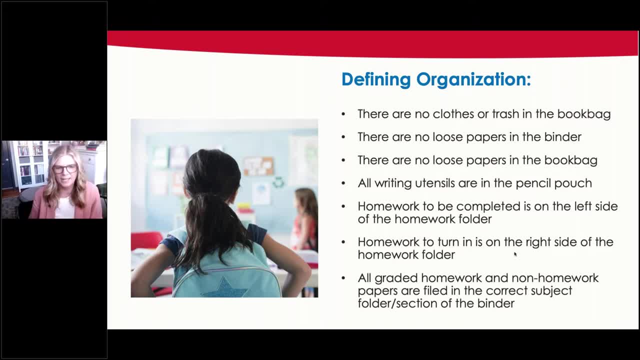 All of your writing utensils are in the pencil pouch and your book bag. You have a homework folder And in the homework folder There's two sides. One's on the left is homework to be completed, and then homework that's done is on the right. 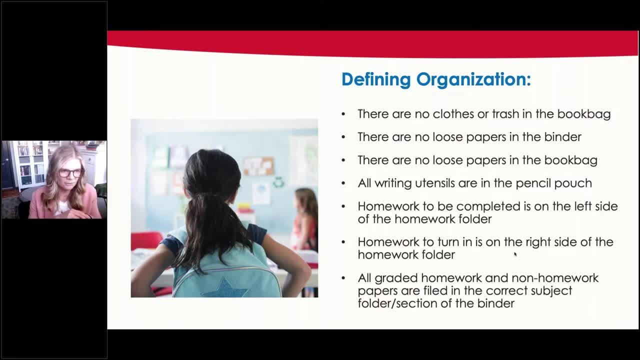 And that other materials that have already been graded or not, in the homework folder, but their files in the correct subject and the binder. So these are some very specific definitions of organization that we would sit down and kind of agree on. what these, what these goals are and 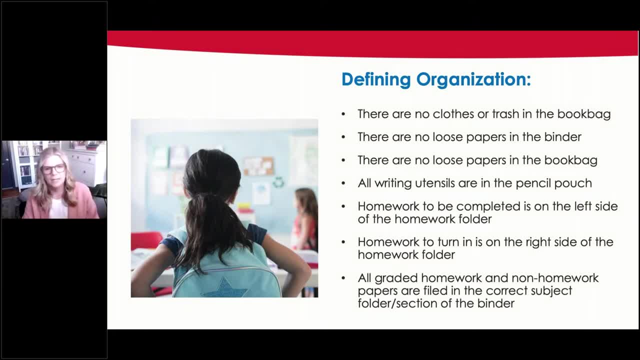 then how this is implemented in the moment is to set up a plan either that the child uses these goals and these definitions of the checklist for themselves to go down and check once or twice a week, or or even more- more is always better- and then setting up a time where the parents or someone in school 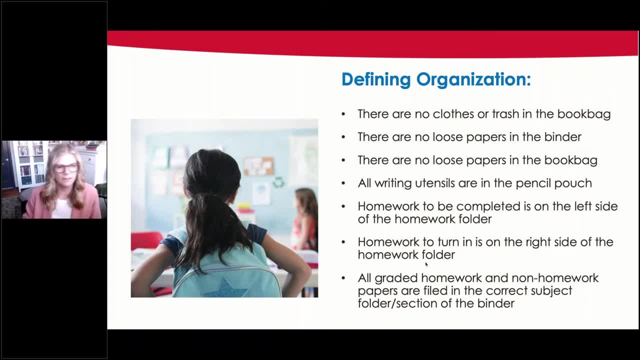 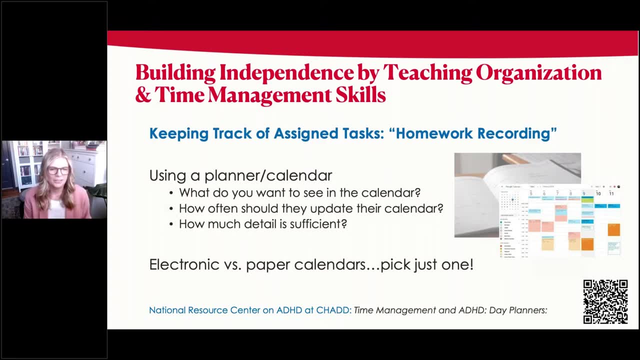 can also check their materials to see if they've kind of checked off each of these goals. okay, so then, moving to another aspect of homework or time management, is the actual homework recording process, or keeping track of what assignments and tasks have been assigned, so using a planner or a. 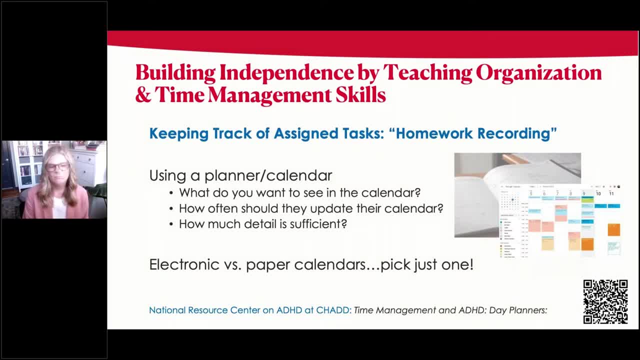 calendar for the student, and there's a variety of different options out there. it used to be that schools would give out planners to all their students. some schools now do that and some schools don't anymore. some students might prefer an electronic system or an electronic system, but there's a variety of options. 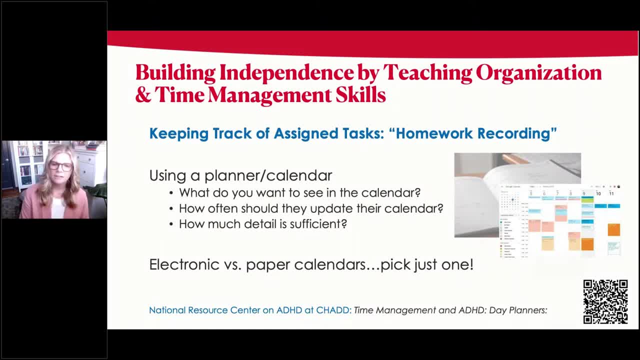 calendar, especially these days, and it doesn't really matter if it's a paper calendar or it's an electronic calendar. There's pros and cons to both, but as long as there's one system that they're using and that they can stick with. Paper calendars are nice if in the school day they're. 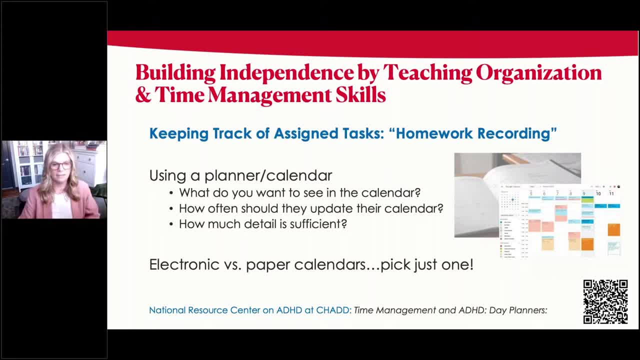 not allowed to have a device or computer up. They can quickly write down assignments when they're moving to the next class or when a teacher brings up something. They have a notebook that they can pull out easily and they can write it down. Electronic calendars are nice, because a parent 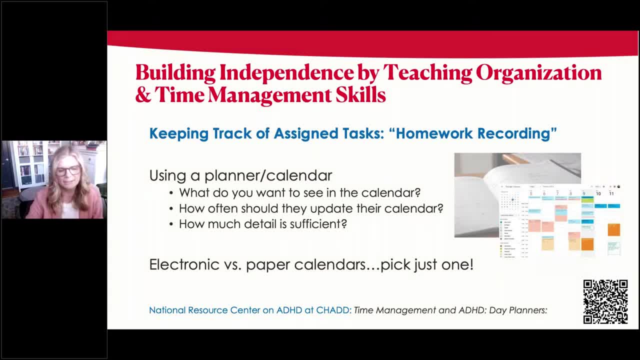 can have the calendar shared with them, They can use color coding systems for different subjects and you can kind of very quickly see a week's day or day zoomed in, And so there's a lot of different features that can be particularly useful for an electronic calendar. So it's just. 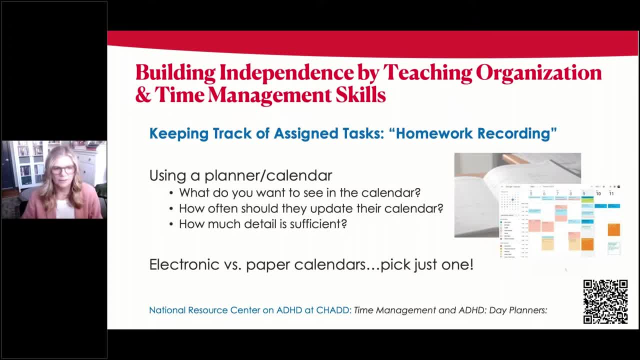 most important that they just pick one and they use one that works for them, rather than trying to do it To juggle using multiple different subsystems. But what we actually work on with using a planner or calendar with students is thinking about how much detail is important. So writing in sufficient. 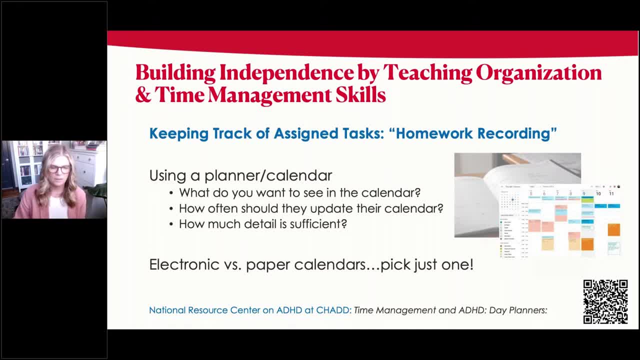 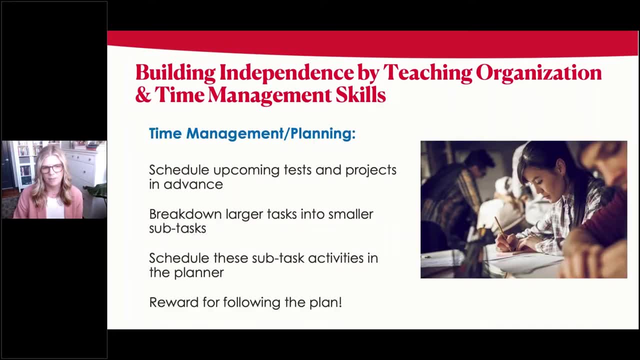 detail, to know exactly what to do, what to study, what chapters and what problems to do. So they're getting points of rewards, rewarding those specific behaviors And then building off of that time management and planning is also sort of using that planner or calendar, but to schedule for. 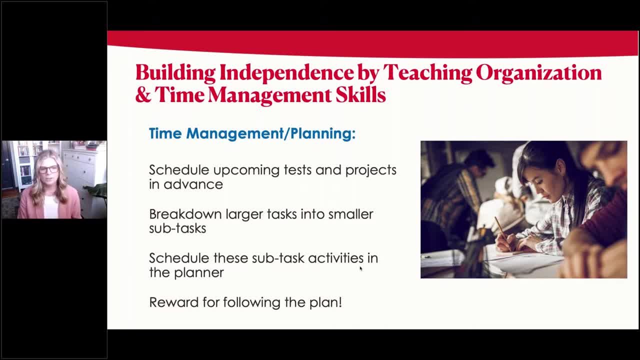 upcoming classes. So that's one of the things that we're doing, And then building off of that planning is also sort of using that planner or calendar, but to schedule for upcoming classes, And here we reward students for adding tests and projects to their calendar, but also for 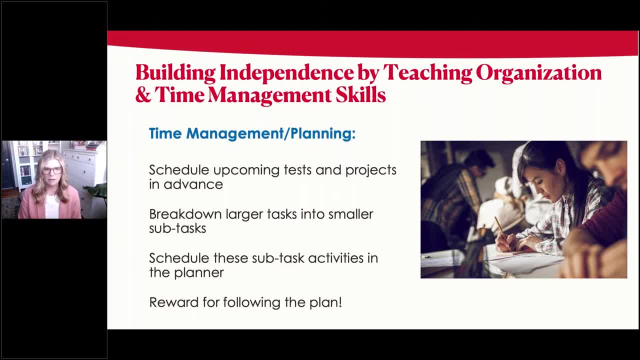 taking the planning steps to break down larger tasks into smaller subtasks that need to be completed, and then scheduling those subtasks into their calendar, And we also focus on sort of specifics of those tasks and what pages they need to do, how much detail is sufficient for these different subtasks, and then we reward them for. 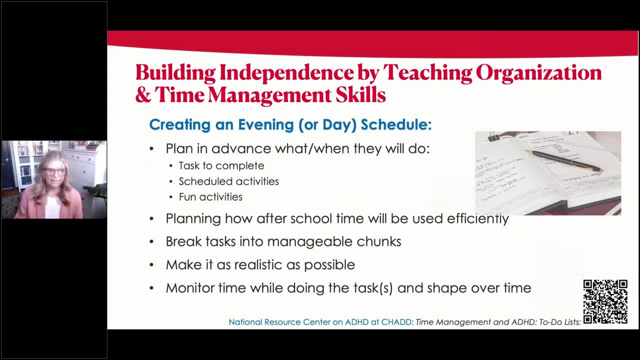 following the plan. Another aspect of planning can be that we create an evening schedule. It's where you resume and look at a single day by the- we often say by at least the half hour increments, not the hour, and helping them first fill in what are the known activities that you. 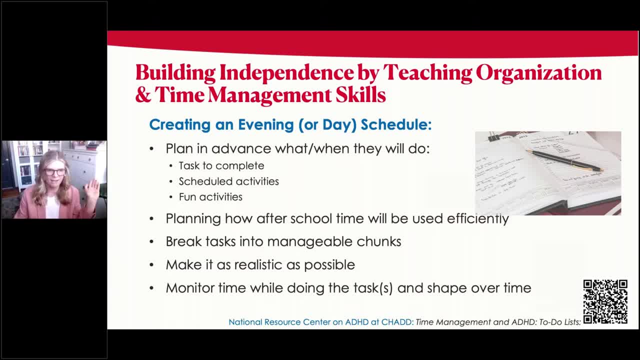 have to do. Well, we have family dinner from six to seven and I have piano practice from four to five, And so then you look back at your planner and what work you need to do and you schedule in your different tasks amongst the spaces that are available between coming home from school and 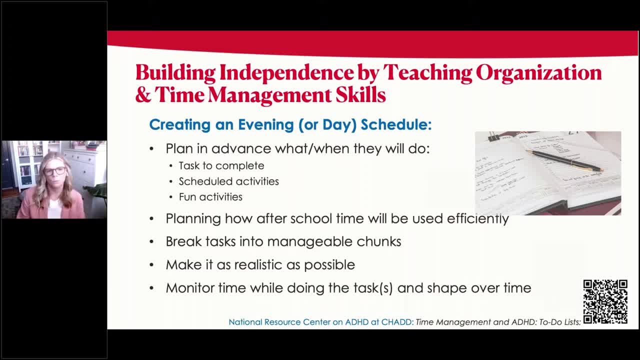 bedtime essentially, and kind of planning around when you want to do what and in what order, how long different tasks take to do. So this is the process of helping them think through planning like their own specific day. We first let them sort of have autonomy and pick when they want to. do the different behaviors, And then we let them sort of have autonomy and pick when they want to do the different behaviors. And then we let them sort of have autonomy and pick when they want to do the different behaviors And then, depending on how that works out, 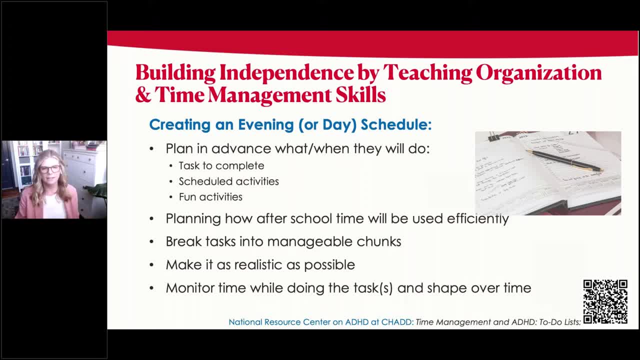 then we'll also perhaps give a little bit more guidance on how did that work? Did your homework after watching your television last time? Was it harder to focus? Did you feel more tired? Why don't this time we try finishing your harder tasks first and then doing your easier tasks later in? 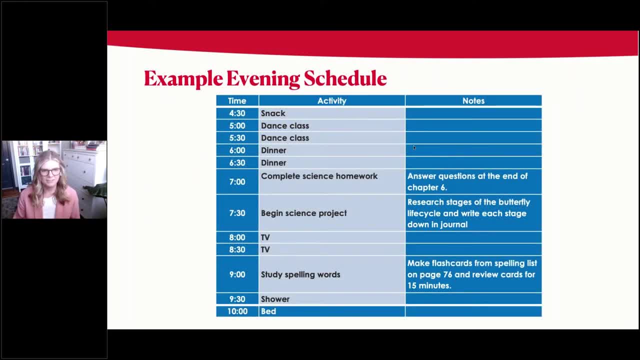 the night. Here's an example of what an evening schedule is. It doesn't have to be in a fancy form or anything like that. It can either just be a zoomed in version of, like a Google calendar, or it can be a blank piece of paper, And then we let them sort of have autonomy and pick when they want to do the different behaviors And then, depending on how that works out, we'll also have autonomy and pick when they want to do the different behaviors. It doesn't have to be in a fancy form or anything like that. It can either just be a zoomed in version of like a Google calendar. 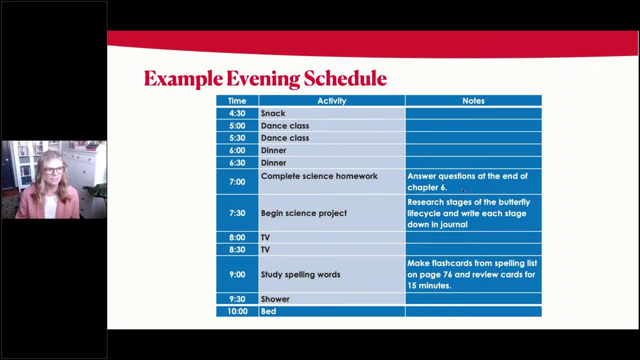 or it can be a blank piece of paper where you write out what activities you're going to do, And then the note side is to write sort of the specifics of what you're going to do. So now I'm going to move into sort of the strategies for parents that really help. 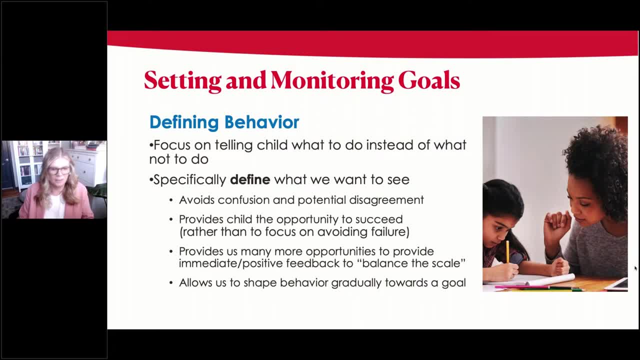 these organization, time management and planning skills particularly work. So these are sort of your global components that make this helpful. These are, these are true for each of these skills. So I mentioned with organizations, defining behavior and the importance of that, And that's really true for all of the skills we need to operationalize, which means to 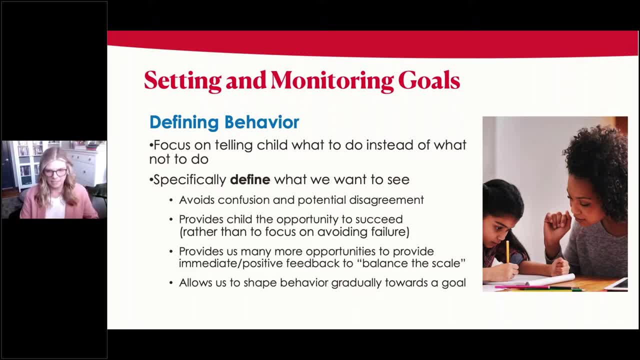 just defining very specifically what the behavior and expectation is, And for some things this can be particularly tricky. So it's good to sort of define it and then test that. we know that everybody agrees on what it looks like. So, talking through sort of what are things that you would be able to? 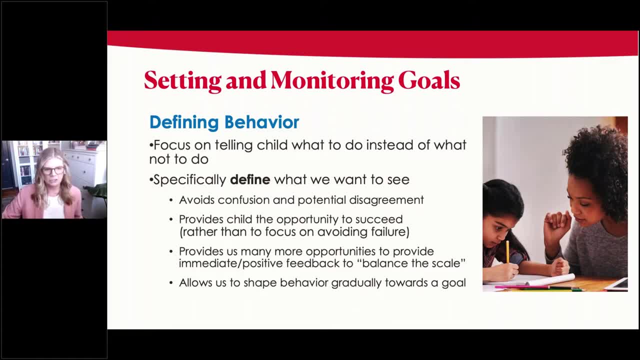 observe and talking through with the child and what they think that that means, and making sure that we're all on the same page. By defining the behavior and setting goals around these behaviors, we're providing opportunities for the student to be successful rather than waiting for them to. 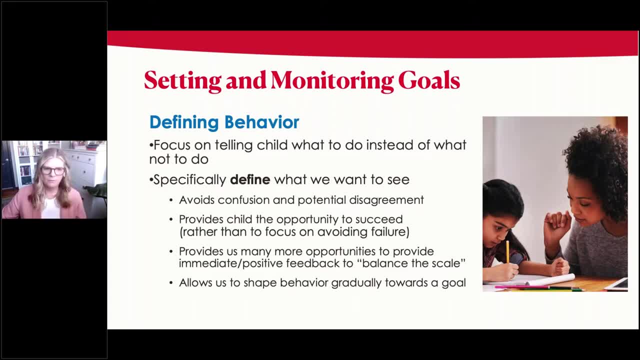 not be successful and then trying to correct that behavior, But instead this is sort of- and as an antecedent or beforehand, focusing on things that they can do and setting small achievable goals around that. The other thing I'll say that's important about setting and. 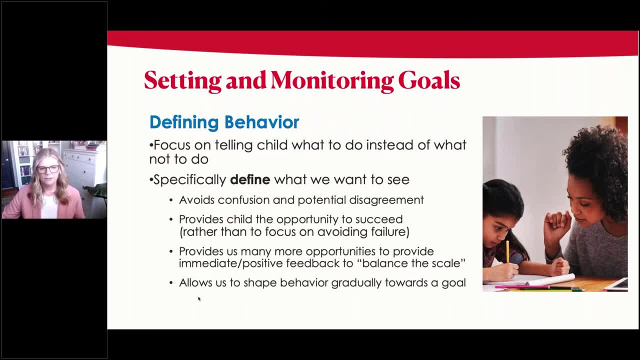 monitoring goals is that- and this is particularly difficult, I think, for families- where it's today and by the end of this week, you want to see that these opportunities are being met, So I think it's important to set goals around that. 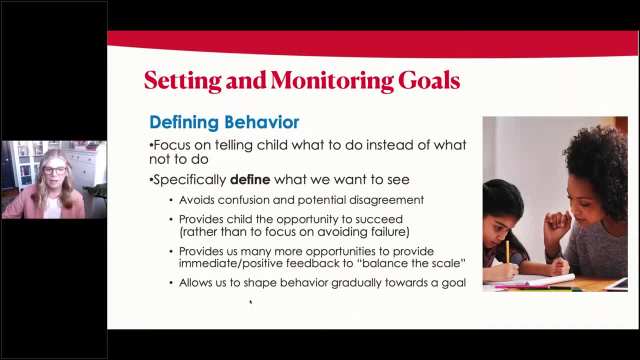 Organization, time management behaviors are just being implemented. The goal of this work is really to gradually shape behavior towards a goal. So if the ultimate goal is to be 100% of the time recording all of their homework, but right now they're really only catching about 60% of their 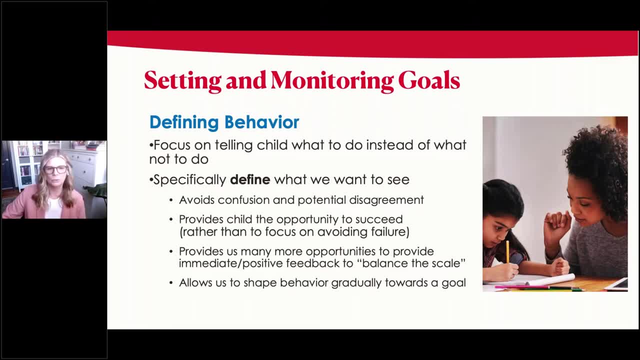 assignments into their planner, then maybe a first goal would be to achieve at least 70% or 75%, And then after a couple week or two maybe we bump it to 85% of their assignments are into the planner And then kind of, you know, we're going to be able to set goals around that. 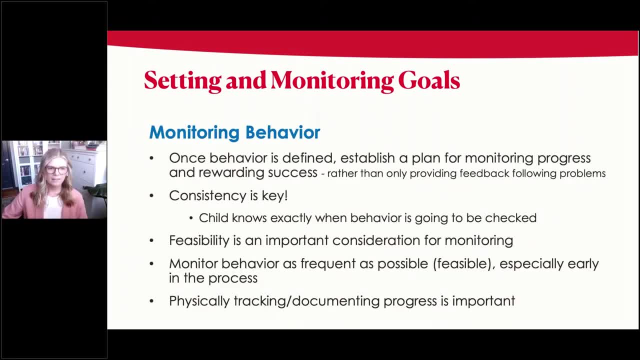 So I think it's important to kind of gradually shape that over time. Once we define the behavior, then we want to establish a plan for monitoring progress and rewarding success. So how often is the parent or if someone's checking in school like a school counselor, how often are they going? 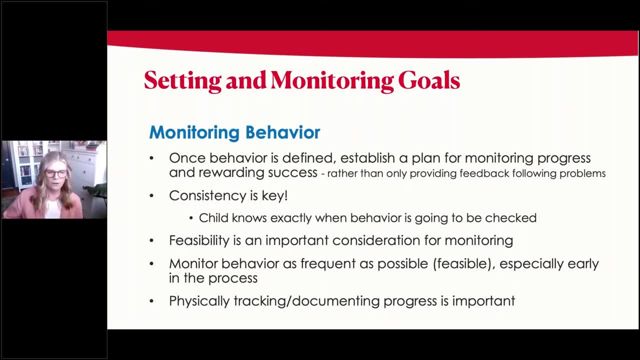 to check and what is feasible or the amount of monitoring that they can do. So setting if parents can monitor once or twice a week and check what are days and times that they're going to do that, And that's a very you know. 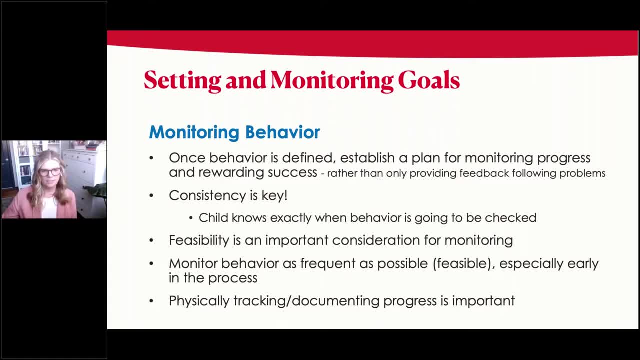 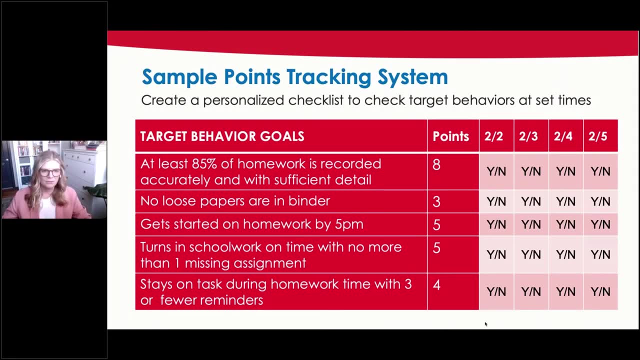 transparent way communicated to the child so they know exactly when they're going to be checked and what days, what times and what the parents going to be looking for. So here's a sample sort of points tracking system that has on here some homework recording goals, some organization goals and some. 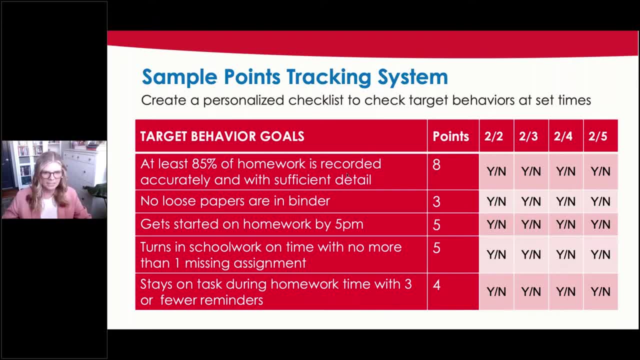 planning goals. Sometimes if we were focusing just on organization we might have five, six or seven goals just on organization. This is a child who had focused on each of those things and now is sort of a person that's jestejuning the last final behaviors, with a few from each area of organization time. 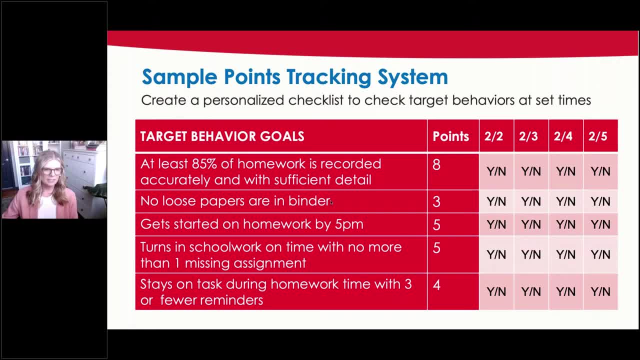 management and homework, and the key idea here is that this is a personalized list, specific goals that this particular child is needing to work on, and they're getting small daily rewards or weekly rewards as well, So that way they can experience success with doing these behaviors and the reason 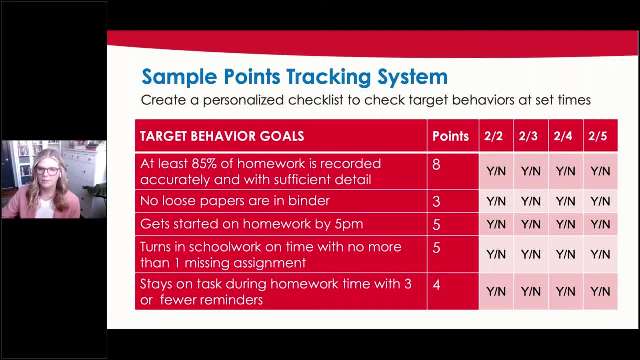 that we have daily rewards And daily reports earned is So that way, when the child makes a mistake- which is bound to happen, especially on youth with ADHD- that they have a reason to kind of be motivated the next day. If they only have long-term rewards and they mess up on one day, then they sort of 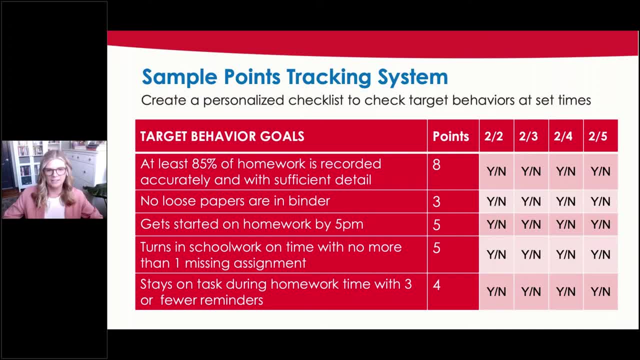 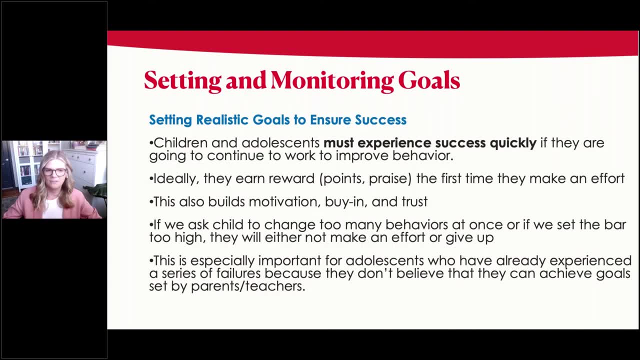 want to give up for the whole week, because what's the point of putting in the effort at this point? So that's why we have both short-term and long-term rewards to kind of keep that momentum and motivation going. I also want students to experience success quickly, And this is important. 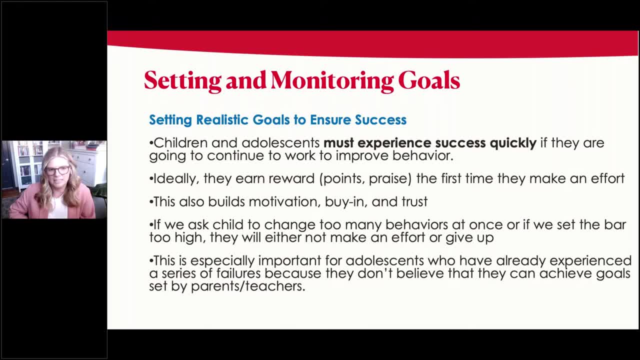 particularly for youth with ADHD who struggle a lot in school. We see this especially for adolescents, who maybe have experienced a series of patterns of trying and failing and trying and failing when it comes to schools or different systems and their academic performance, And so they don't believe that they can achieve the goals that are set by their parents. 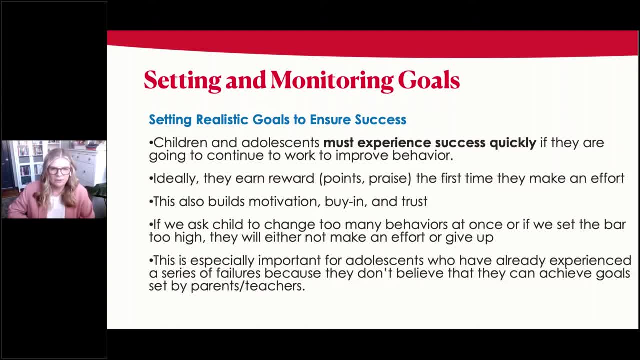 and their teachers. So we need to start small And that's why we start with just a little step above where they currently are, even if to a parent doesn't feel like it's making much progress. When they experience that success we're building an internal intrinsic motivation to do these. 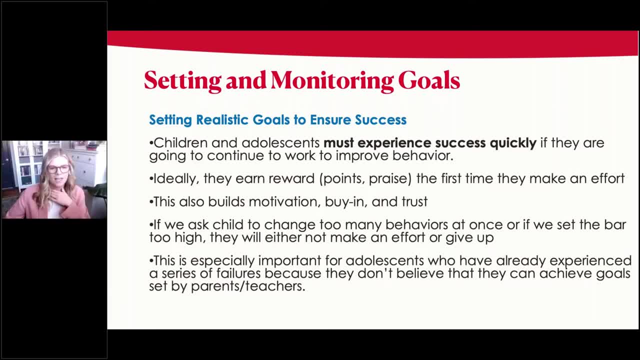 things, because when we feel that we're good at something or that we can be successful with something, we're more likely to keep working at it, And so if we set the bar too high, then we're just reinforcing everything that they've already experienced, which is that this is too hard. I'm 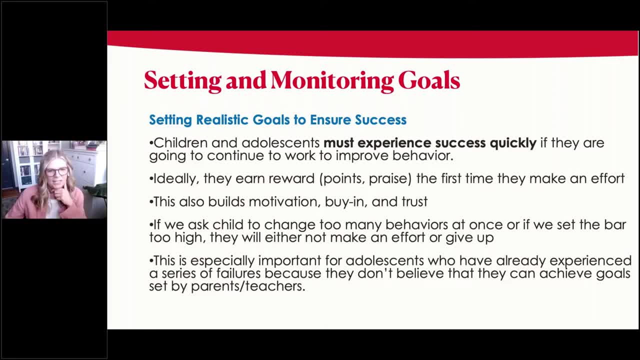 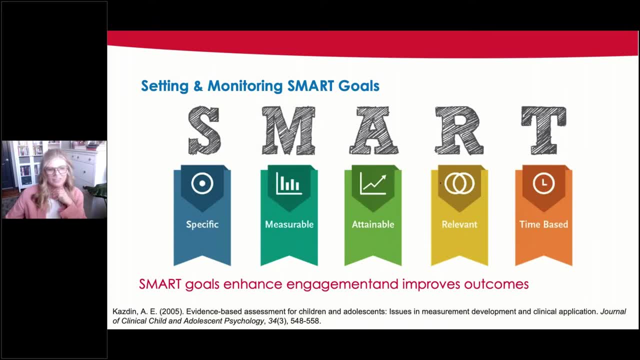 going to give up and there's no point in making any efforts. So that's why we sort of try to set the bar low, get their buy-in and their motivation. So that's where we're going to start really early on and then take it from there. 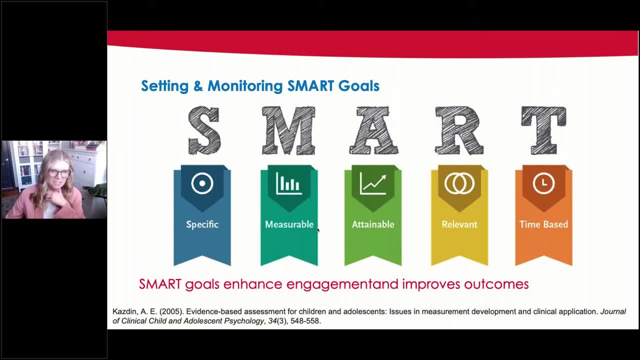 Here's just a little infographic on SMART goals. This isn't specific to homework, organization, time management interventions. It's an acronym that's used in a lot of different programs around setting goals, but it's a good reminder when you're setting these goals that they should be. 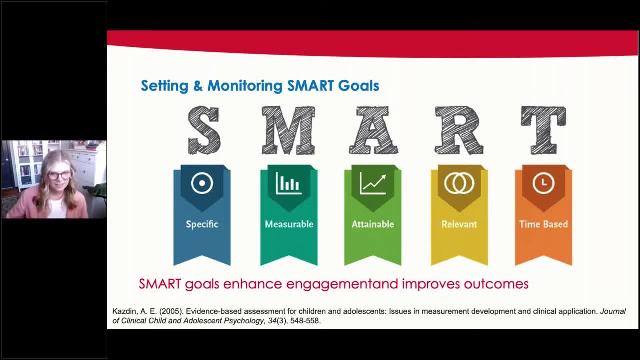 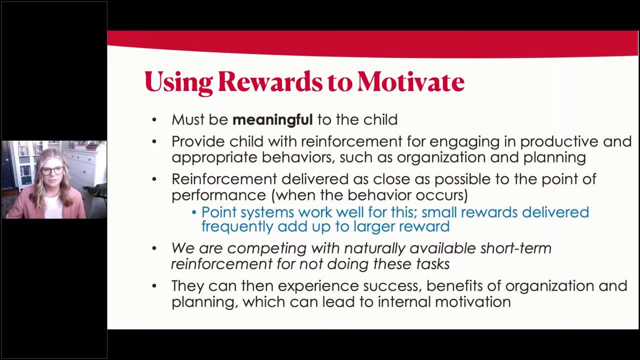 specific, measurable, attainable, achievable, relevant to that child or individual and time-based. that we know kind of when we use rewards to motivate the child for doing these target behaviors. and that's where we're going to start. So we're going to start with the rewards. The rewards are really important, Point systems can. 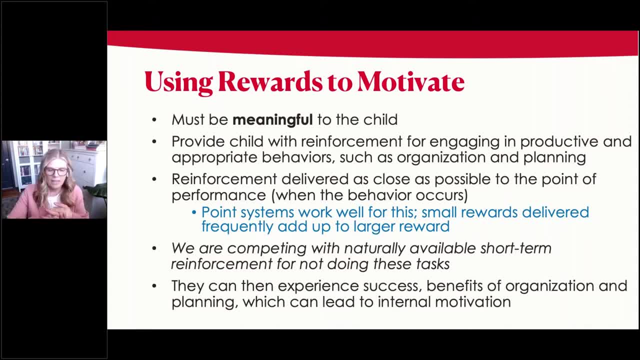 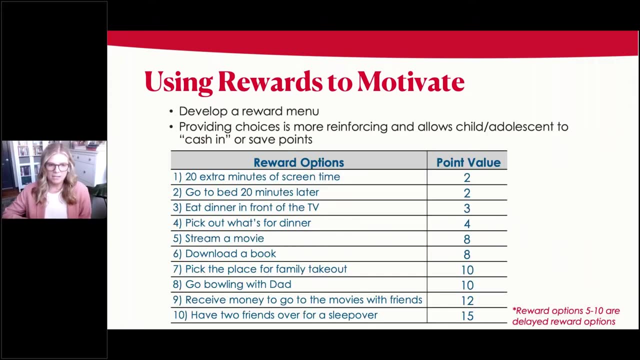 be especially well for kind of tracking the behaviors that are done and the rewards that should be delivered. As I mentioned, they should be given frequently and they can add up to larger rewards. but we want both short-term and long-term rewards, So we like to use a rewards menu. 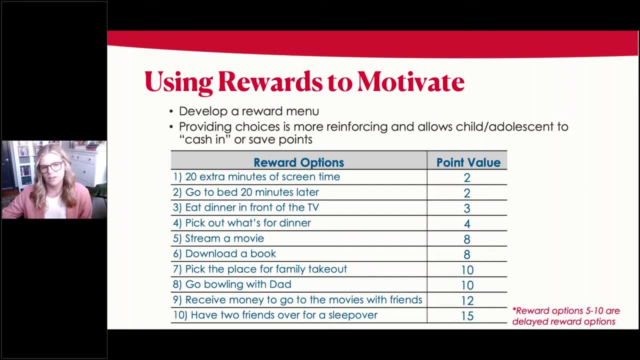 and this is something that should be developed with your child- where they add things to it. You can brainstorm ahead of time. What are some things that you're willing to put in here And where do you draw the line? But you'll see there's different point values. So some things. 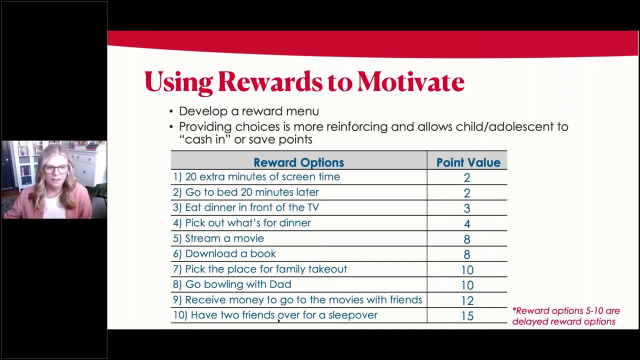 the bottom half of this table are things that are going to require a little bit more, So maybe they have to be done on weekends. So these are longer term goals, So they have the option of cashing in or saving up. Then we like to set a plan, So we want to sit down and sometimes we can call this a 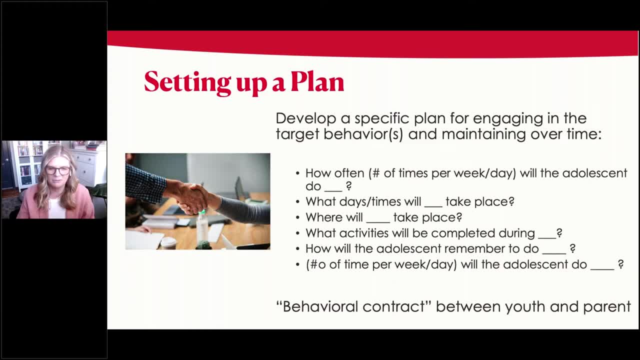 behavioral contract. Some for younger kids maybe don't like that term, but it's really just a plan For both parties, both the parent and the child. what you're going to do, how you want to be reminded, are you and when is the parent going to check these behaviors? Where's it going to occur? 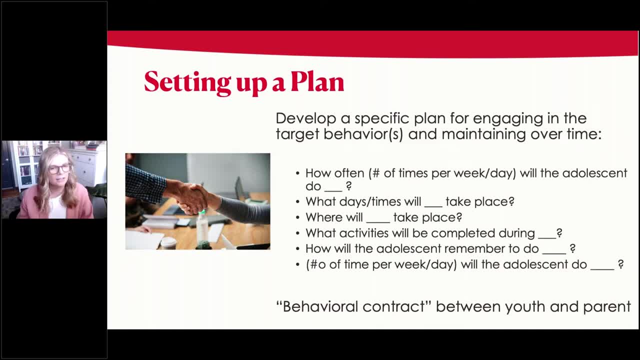 And this is so. that way, everyone agrees to what you're going to do. If the child says no, I'm going to set alarms in my phone. I don't want my parent to remind me, Then it's the parent's job not to be asking them about it throughout the week. Okay, the last point I want to make is: 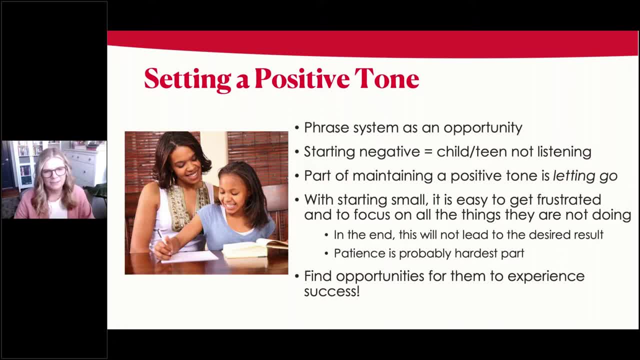 setting a positive tone. This is so important. So, if you're a parent and you're going to be working with a child on a day to day basis, what is there for you to learn to do? I think it's really important. As I was saying earlier, there's school and academic behaviors. 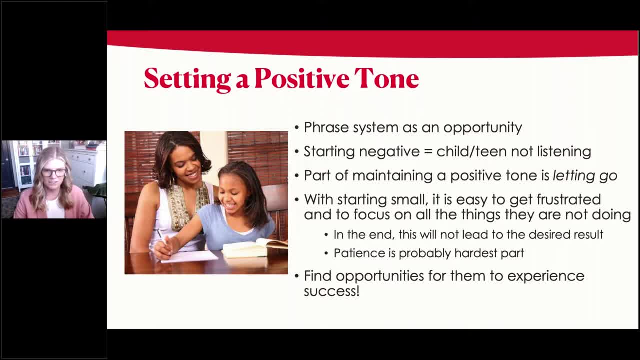 and academic efforts when it comes to youth with ADHD is often a struggle, And so it's really important that we introduced a new system, that we phrase this as an opportunity. If we start with the negative, we are already just risking the child or the teen just not listening. So if we 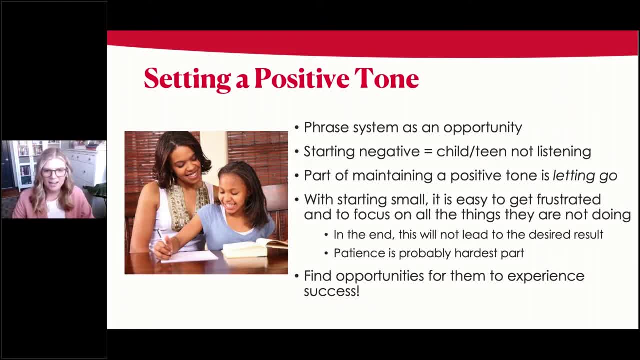 were to say something like: you know, you have been procrastinating a lot and this is a chance for you to take a step back and start over, And so that's really important. And, as I was saying earlier, there's school and academic behaviors, and academic efforts when it comes to youth with ADHD is often a 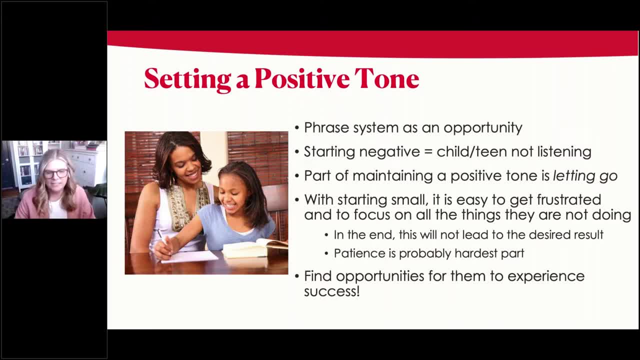 is just really becoming a problem and we need to do something about it. Sort of this has this negative tone and immediately they're going to just, you know, drone you out. But if we start with a different way, like approach it, such as I can remember when I was in middle school and 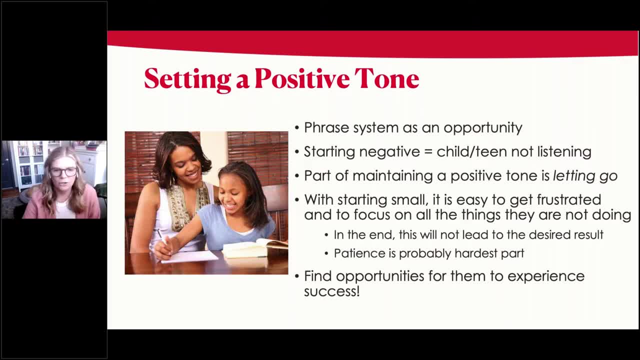 it's a lot to manage multiple teachers and I know you're working really hard to improve your organization and record your homework And so I want to set up a system with you where we reward you for those efforts and really reinforce all that you're doing to try to improve So that sort. 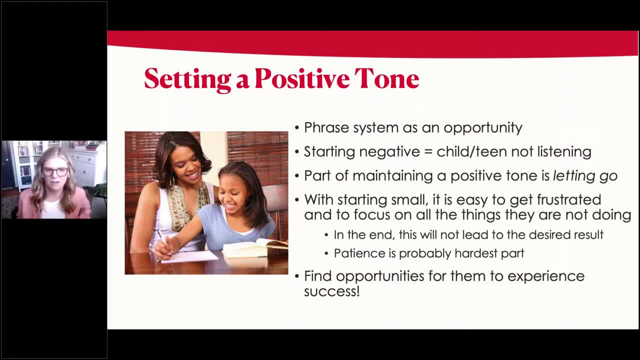 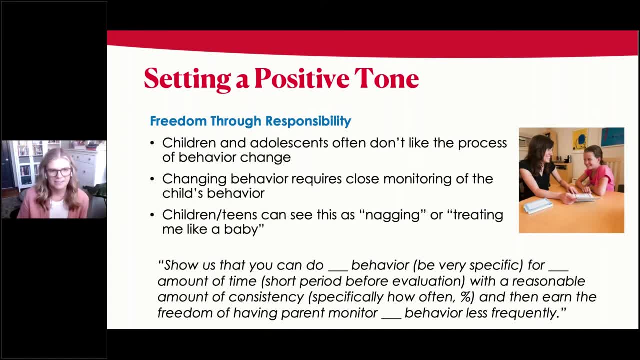 of sets it up in a more of a positive tone and maybe perks their ears around getting opportunities to be rewarded for their efforts that they're doing. And here I just sort of put at the bottom of this sort of an example of that text: So show us that you can do whatever this behavior for X. 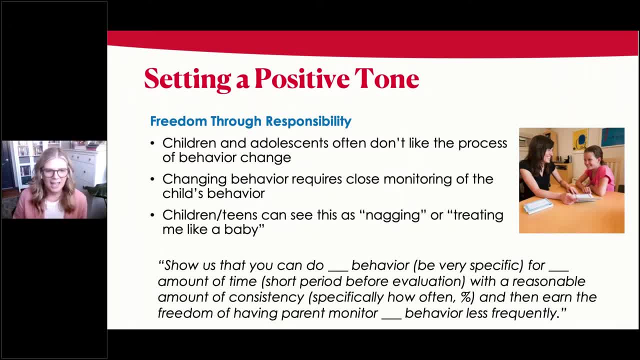 amount of time with a reasonable amount of consistency, and then they can earn the freedom of having their parent monitor. So this freedom through responsibility is something for children and adolescents. When you introduce new systems, sometimes they really don't like having all this increased monitoring from a 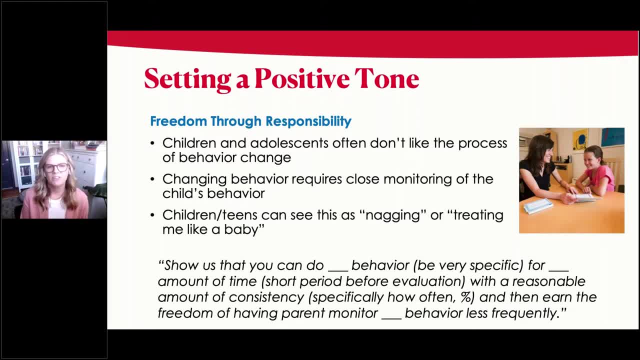 parent or a teacher or someone at school might make them feel like a baby or a young kid, And so we phrase this as sort of: the more that you demonstrate that you can do this on your own or independently and gradually over time, then the less monitoring that you'll have, And that ends up. 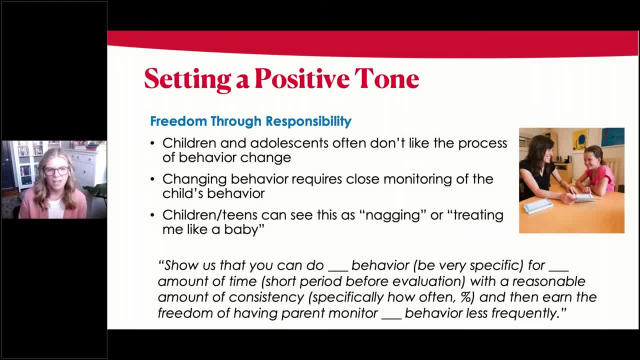 being kind of, quite, you know a little bit more of a, you know a little bit more of a powerful reinforcer on its own, sort of getting your parents off of your back or sort of getting more independence in this area. So we focus on that with a positive tone. And then, lastly, I'll 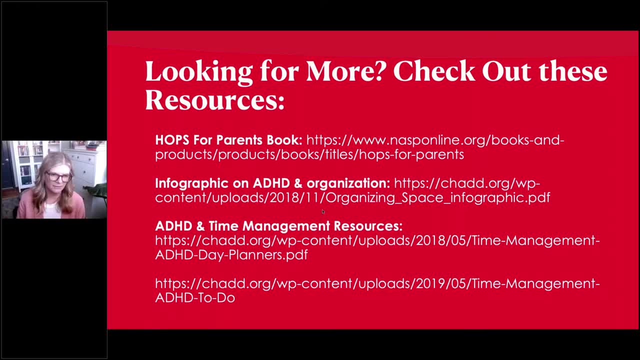 just put up here some resources for parents. There's a lot of really helpful materials on the Chad website when it comes to different infographics and tips for homework and time management. Here's a link to the HOPPS parents book that's available for parents. 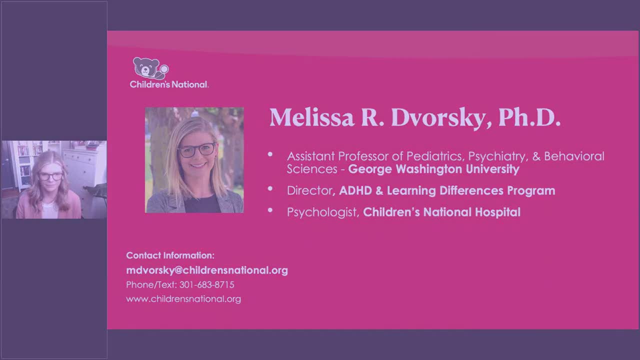 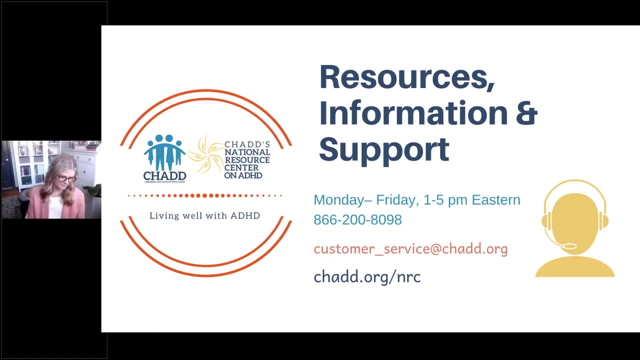 And lastly, there's my information if anyone wants to reach out and contact. At what point do you seek counseling for CBT, for difficulty in attaining motivating themselves? That's a great question. Thank you for that question. For any of those that aren't, I'm sure. 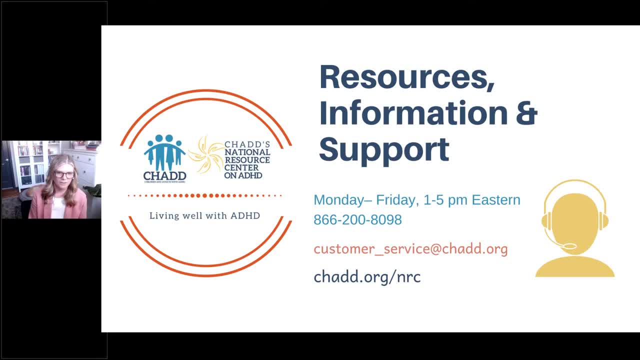 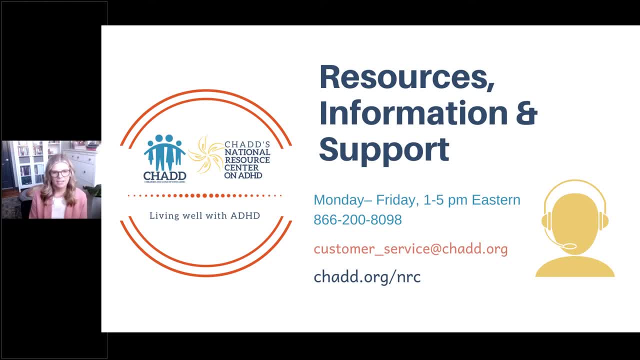 And it can be useful for adolescents with ADHD when they are experiencing difficulties with motivation, especially if there's other mental health concerns such as anxiety, stress, mood or depressive symptoms. CBT or cognitive behavior therapy can be really helpful for that And in 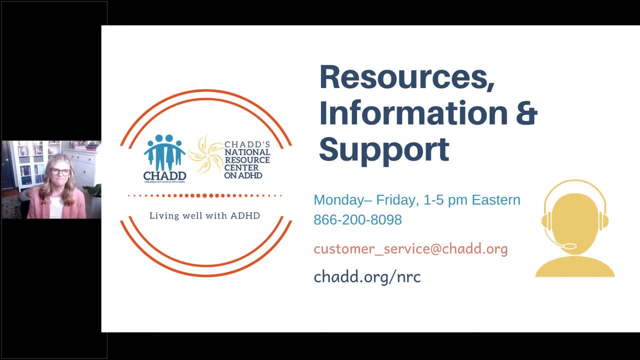 terms of addressing kind of when and when is it important to kind of go and seek help for that? that's sort of a tricky question to just there's no like clear cut rule on that. But if you feel like you've tried some of these strategies and it's very difficult, or you as a parent on your 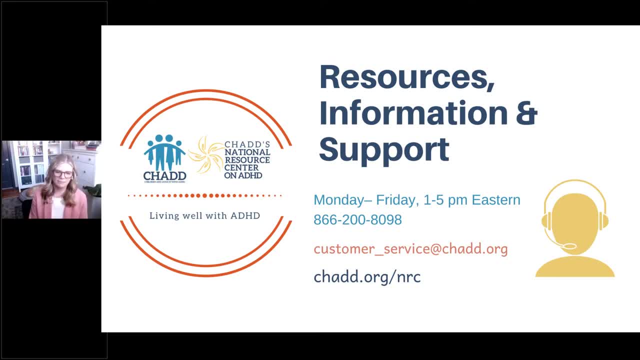 own to be motivating them and you've tried setting a positive tone and starting small goals to work towards to motivate them and still really struggling and noticing that there's additional sort of mental health either concerns or you know potential areas where they might be struggling, then it's certainly helpful to to seek help And 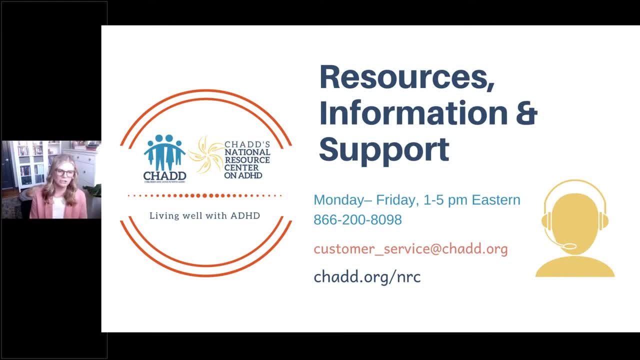 you can always something that you can talk to your doctor about your primary care doctor, where you could seek out- you know- different mental health providers in your area to see whether that's something that could be beneficial to you- learn about what that would. 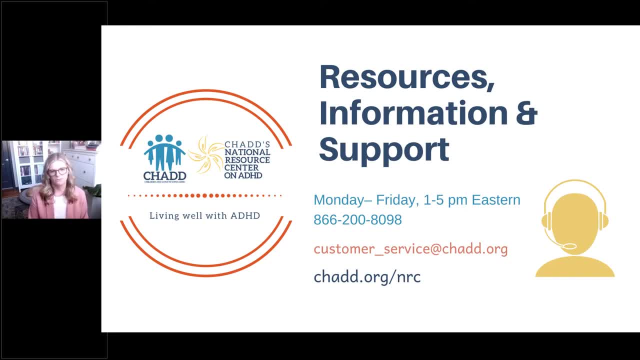 look like what they would do and see if that's something that could be helpful for your child. Do you have a recommendation for a specific how to guide for setting up a point system? The details are often important and many parent resources just tell you to do it but don't necessarily tell you how. 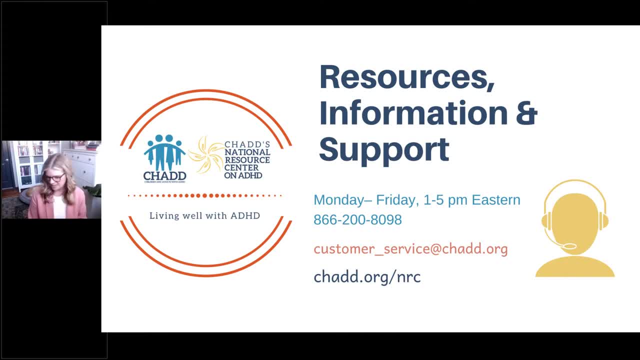 That's a great question. Thank you for for that. That's helpful to hear And I think you're right. A lot of them, a lot of resources you'll see, are kind of vague out there of how to do it, And maybe the reason for that is is that it really should be personalized. So, reflecting back on some of the points that I made today, 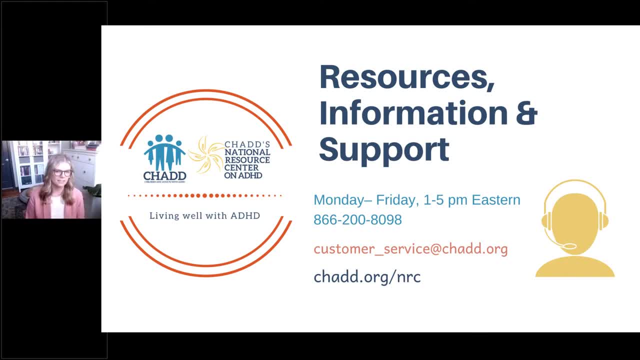 they should be behaviors that match whatever your child's behaviors will be or your adolescent needs are. and thinking of that homework cycle, whether it focuses more on organization, homework, actual completing tasks and staying on focused, or planning ahead for things, so it can have different sort of targets in there, but I think the important thing is that whatever 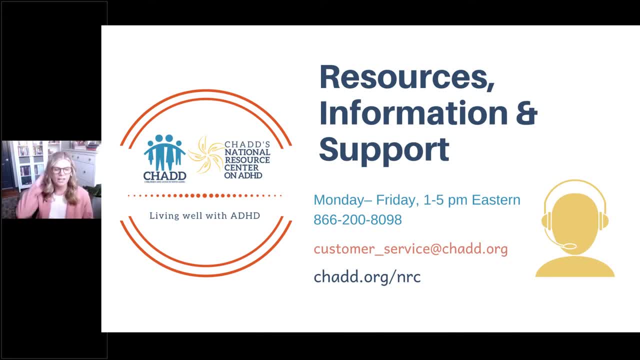 the behaviors, the targets, the goals are that you're earning points for that. they are specific, that they're measurable. so they're things that you can observe and you know there's certain set times when they can happen or they can happen by. so we want the behaviors to be specific. they need 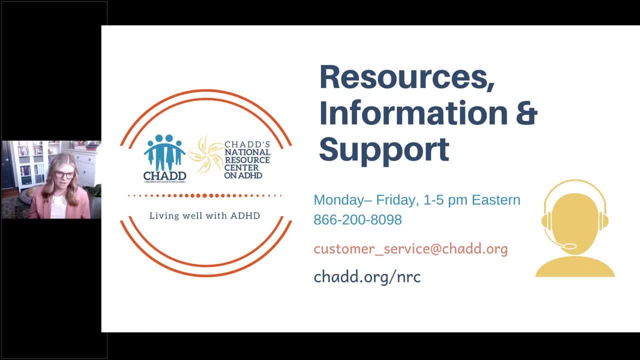 to address sort of the things that your child's needs to work on and they need to be achievable. so we usually like, especially early on, when first doing a point system with your, with your child. we want them to experience success with it, so they need to be able to earn a reward, even if they 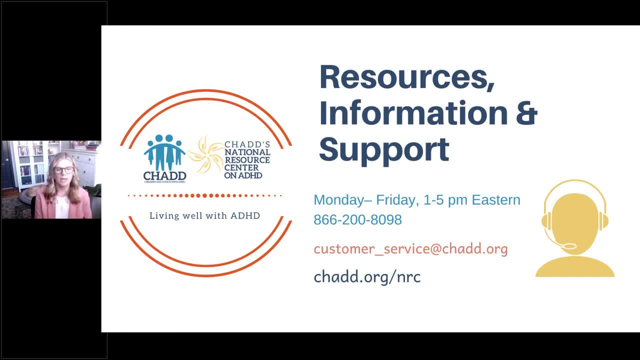 don't have a perfect day where they earn all the points, and especially youth with ADHD, we wouldn't expect that to earn 100% of the points all the time, and not in the beginning. so we set goals, with some of them being ones that we are pretty positive they're going to achieve, and then some of them might be. 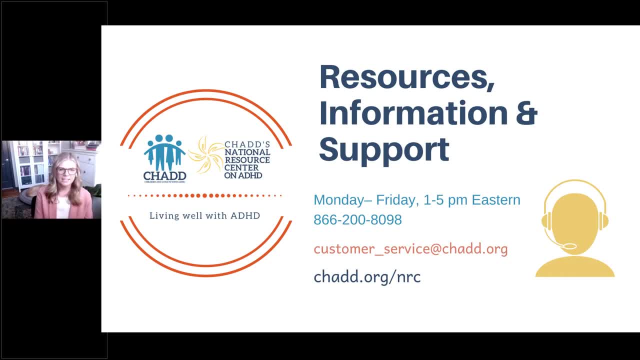 a little bit harder for them to achieve and this can be the hardest part for families- more parents- because it really requires a lot of patience to set goals around things, some things that might feel weird- that setting a bar so low in the beginning, but we do really want to make sure. 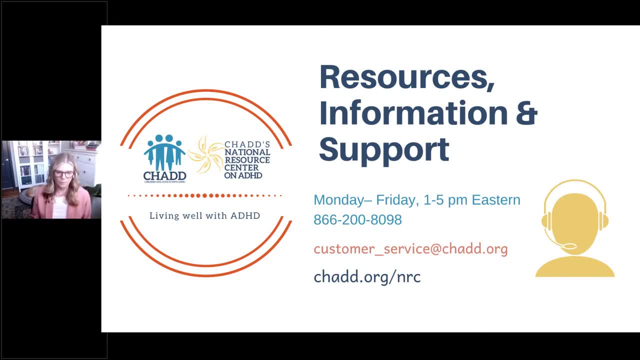 that they're having success. so they are motivated by- you've been using their point system at all, so setting achievable goals and then tying those points to something that the adolescent or the child cares about. so I'd say sometimes of really young children, they can be motivated by just getting that sticker on the. 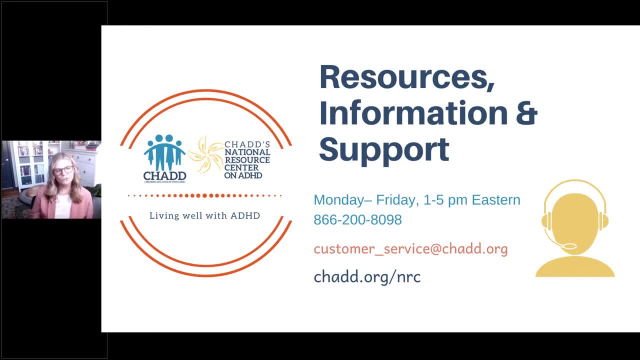 points chart or a star color filled in older youth- their older and adolescents kind of need those points than to translate certain privileges or rewards that they can earn, because the star itself might not be as motivating the older adults who are there. so it's gonna be a lot harder when kids get involved with their parents, but every person who is involved with it just feels like they have certain privileges or rewards that they can earn, because the star itself might not be as motivating the older adults who feel like they're just doing an eighto there, to tell them they're just doing a 10-day. 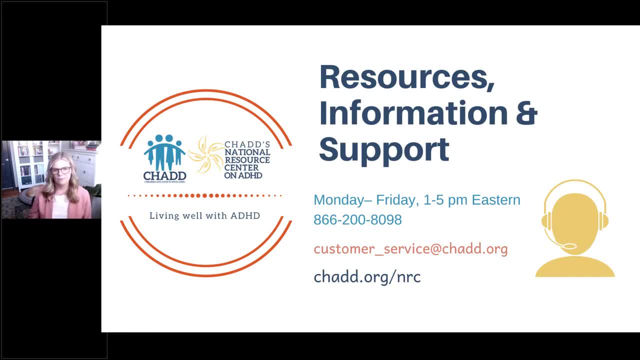 older, they get so tying it to things that they they care about. they're motivated by and having a reward menu, so that way they have options to choose from and that menu can always change. it's hard to suggest any one given menu or reward for child, because what's motivating to children? 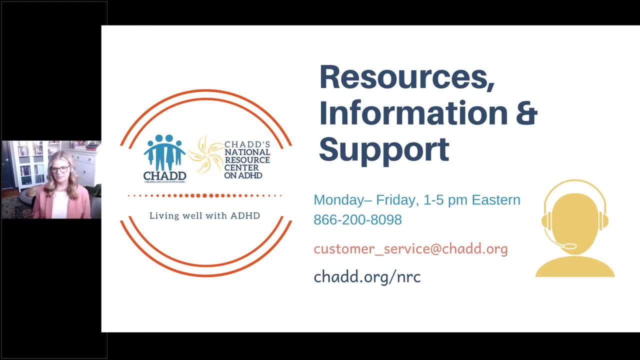 today, it's that's not cool tomorrow. so sometimes I don't put specific things up. for that reason. those are kind of the core things: making sure that it's specific behaviors, that it's something that can be feasibly checked and that you agree on ahead of time. are we going to check this every? 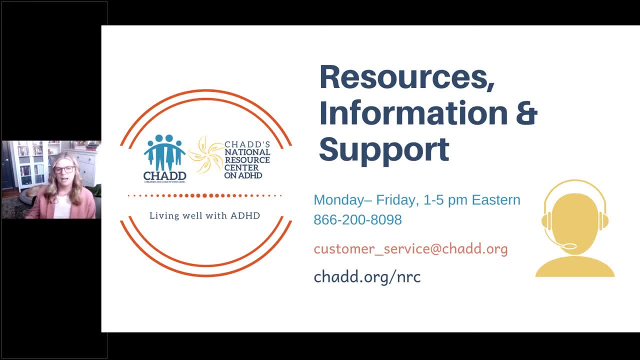 day, are we going to check this once a week? but, being consistent, and however often you set out to do it, those goals are achievable and that it that it's goals that they can. they can still earn rewards even when they have. we want to make sure that they earn those rewards initially, in starting. 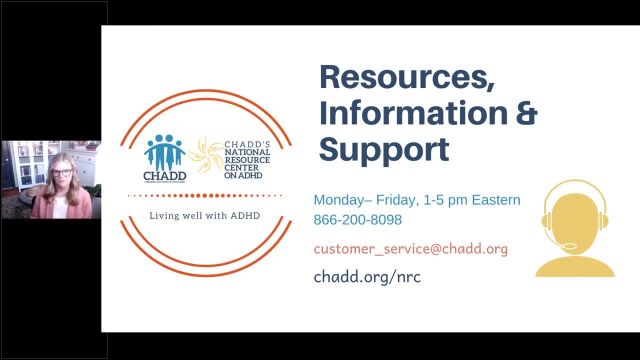 it and that the goals are achievable so they can earn the rewards. to be motivated, do you have any suggestions for the child who says that they have it all under control but really doesn't. they don't want the help but clearly could use some coaching on organizing their time and organizing their work. yeah, that is very common, I would say, and sort of. 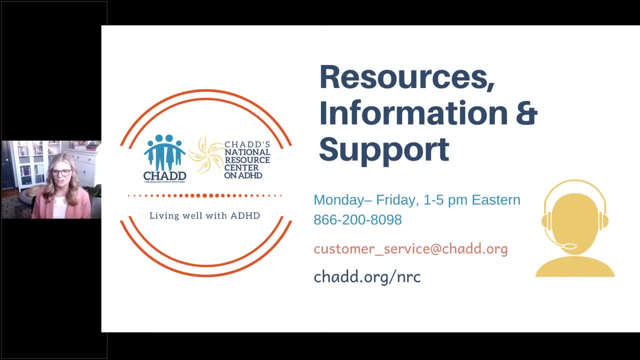 developmentally appropriate for adolescents or older students to say things like that, because they are going through a place in their own development where they are growing in their autonomy and feeling like they're going to be able to do it, and they're going to be able to. 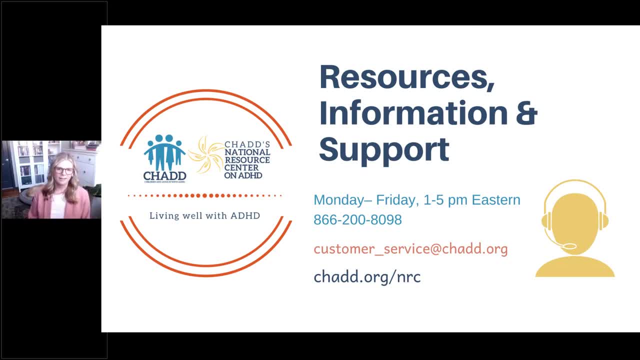 do it independently and take pride in kind of doing things independently without others help the older they get, and so it's important to sort of respect that autonomy and that independence. but if it's obvious that it's not working out, just because they say they've got it and doesn't. 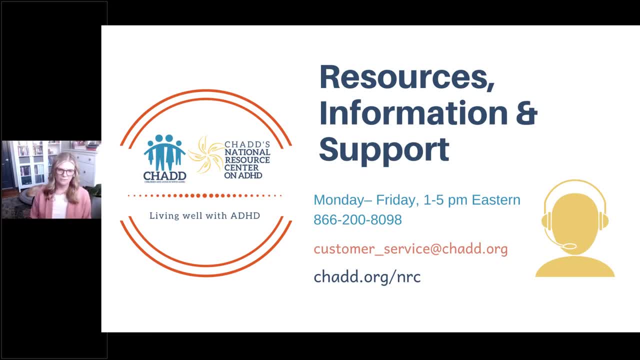 necessarily mean that we should take their word, that they have it under control if there's no evidence that they do so. sometimes one way that I will approach this is sort of setting very concrete sort of next steps, and I think that's a really important thing to do is to sort of 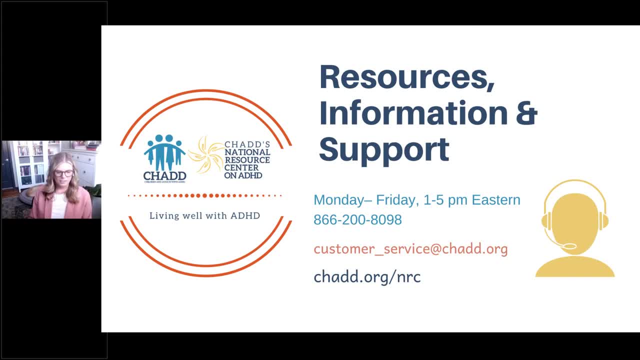 step around this. so, okay, you say that you're on top of your organization. if you don't lose anything in the next week, then I will keep doing it your way, but if you do lose something in the next week, then I'm going to suggest that we try. we just try out doing this a different way, and then we talk. 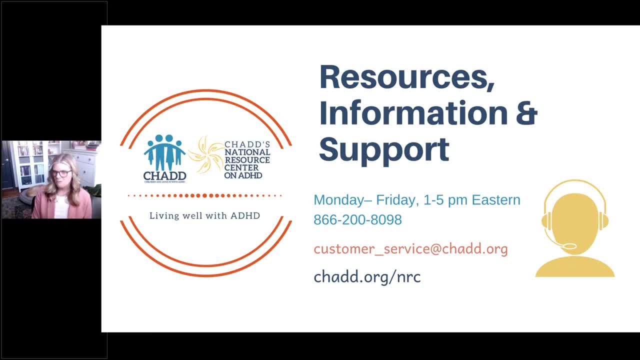 about how we can approach that, or maybe it's. I don't need help with my homework recording. I might first allow a little time to do that, and then I'll do it my way, and then I'll do it my way and then I'm like I'd say: no more than a week of them. okay, let's do it your way and let's see how it goes. 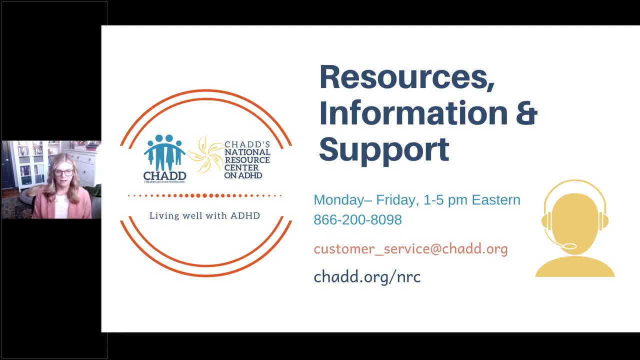 and then that way you kind of get their buy-in on whether that worked out or not. sometimes that's one approach that can work. other times you could, if you think it's too critical to sort of wait and then assess, you could always go the route of saying something, like you know, I know that. 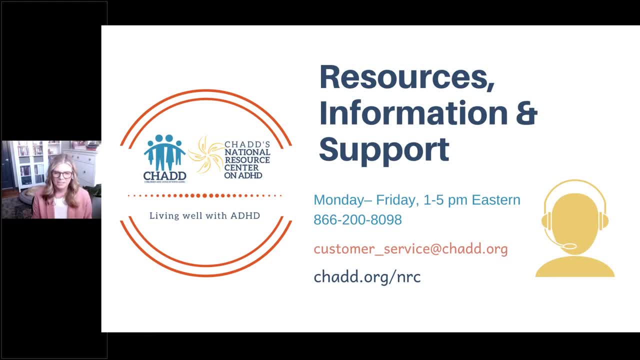 you're working really hard to do this and I- my goal isn't to be nagging you- and so I wanted to set up a system that would work for me. and then I would say: no more than a week of them, okay, let's do it my way. and then I'd say: no more than a week of them, okay, let's do it my way. and then I would say: 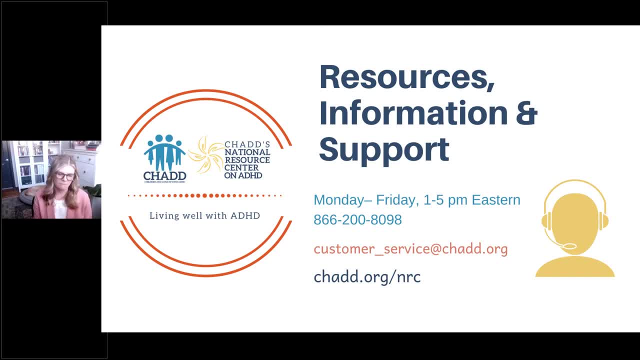 no more than a week of them. okay, let's do it my way. and then I would say: no more than a week of them where you kind of help define with me what it means to be organized or what it means to be homework, so that way I, instead of me getting on you about this, I can be giving you rewards to. 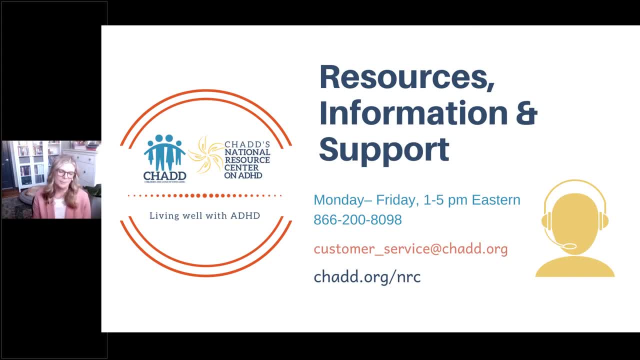 encourage the efforts that you're doing, so kind of phrase it as an opportunity to reward them, because I think youth who want to kind of do it on their own and not be bothered by it are really looking to just sort of get- get their parents off their back or get- um, not be nagged. 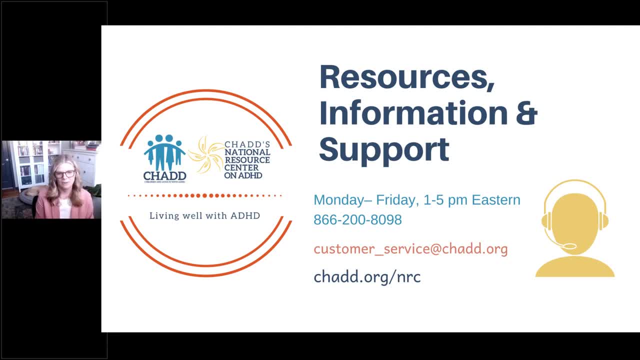 about it all the time. that might not necessarily mean that they're not going to be able to do it and that they need the help, and so that's one way to kind of phrase it, as an opportunity to reward them for the efforts that they are doing, kind of not acknowledging the fact that maybe they might 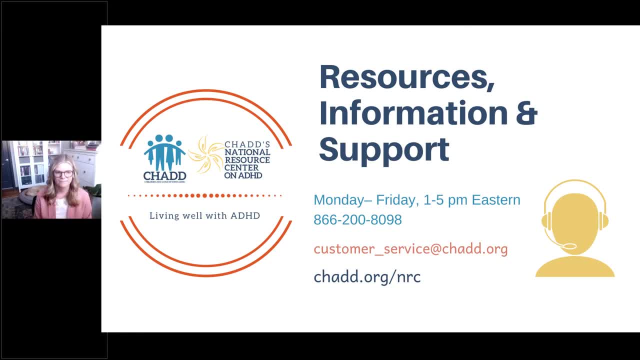 be doing some of those things that you wish they were for younger kids, mainly like eight to ten, would do you think that an ADHD coach would be helpful to prepare them to prep for middle school and some of those added pressures? it sort of depends on their school. I was talking earlier. 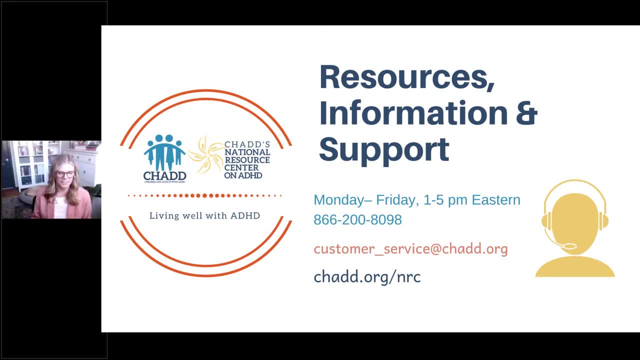 about sort of middle, the transition to middle school, being a good opportunity for learning um organization and time management strategies. it sort of depends on if they have enough work or projects that they can actually plan ahead for or manage their time for, sometimes depending on the student, school and what homework kind of they're getting at age eight to ten. 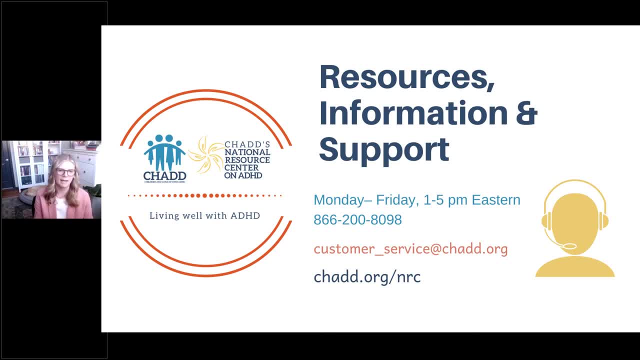 sometimes that's a little too young to be to practice some of those skills. we wouldn't expect them to have those skills yet, but they certainly come online in middle school and there's just. it sort of just depends on the school and whether there's opportunities to do that, but I think 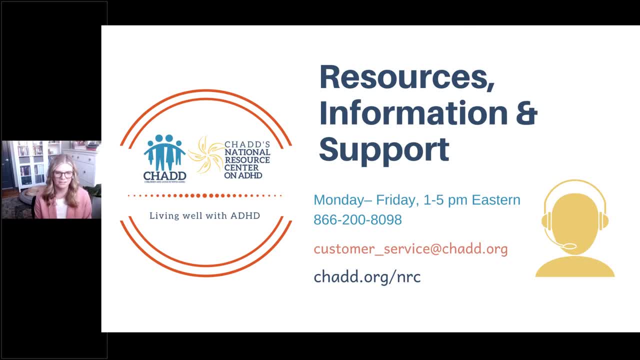 it's certainly. it's always great to get in the habit of doing these strategies and practicing before there's a problem or in a problem area to identify it, and so it can be good to kind of develop these habits early on, but sort of depends the strategies that you have shared. 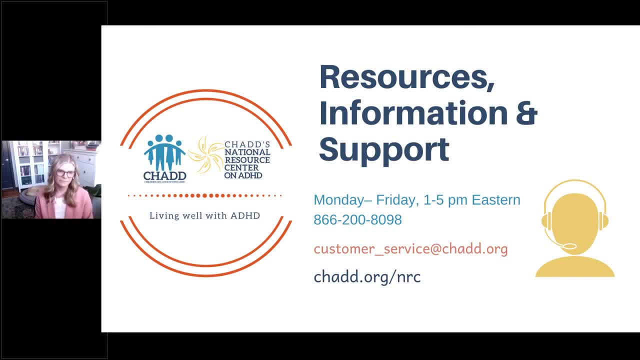 today. have you found them to be effective for children who have both ASD and ADHD? that's a great question. so my work and research. I have not looked at samples of youth with ASD and ADHD, but there are actually other folks at Children's National where I work that do that. 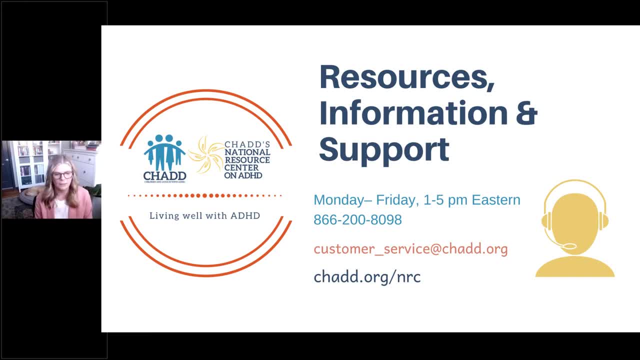 specific area and the intervention strategies are very similar. They focus on encouraging these organization, time management and strategy skills. So not in my own specific work have I found that, but yes, there is a great deal out there and it's very similar. That's a great. 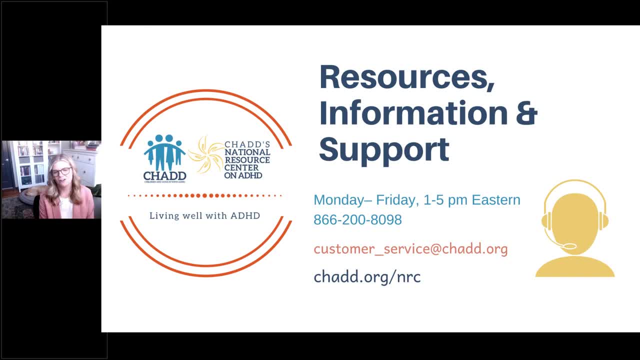 question And chapter reading can be difficult for youth with ADHD if, depending on the subject of that they're reading, if that's something that's interesting to them or not. As you might know, certain subjects in school are harder to get through that homework assignment than others. 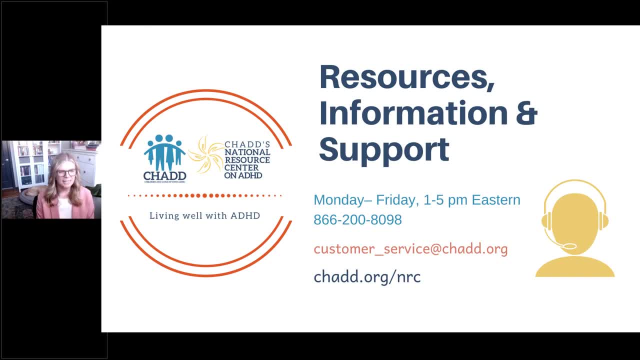 might be more easier if they're fun or they like that subject. And reading can be like that too And I think as adults you can agree. you know, if you're liking the content it can be fun to kind of get through and pass the time and you wouldn't even know it. But then other subjects. 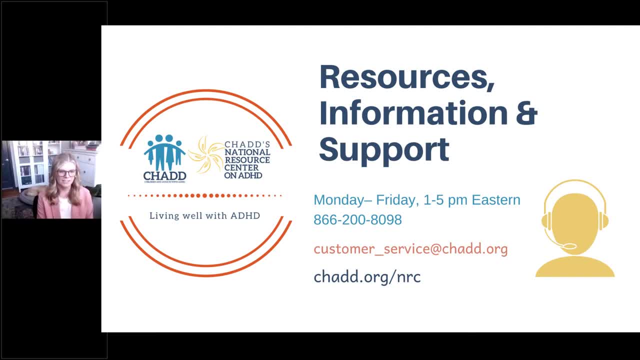 it can be really hard to sort of get through reading that material or that entire chapter. So we like to recommend a few things. One is you can use a timer. Timers can be helpful for sort of setting goals around how long you're going to read and stay on task with your reading. 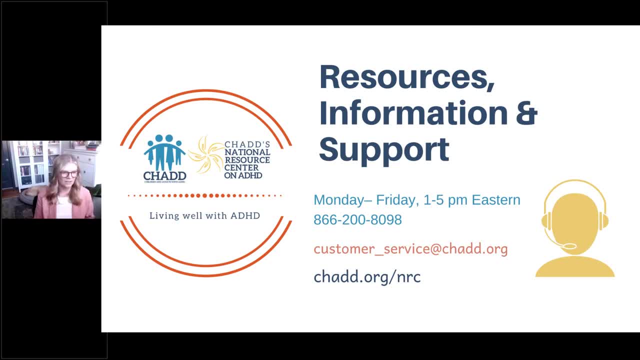 and sort of starting small. If right now they can only read for a couple of minutes before they start getting distracted, then maybe set the goal around two minutes, five minutes, 10 minutes. it kind of depends on their age range and where they're at and kind of work. 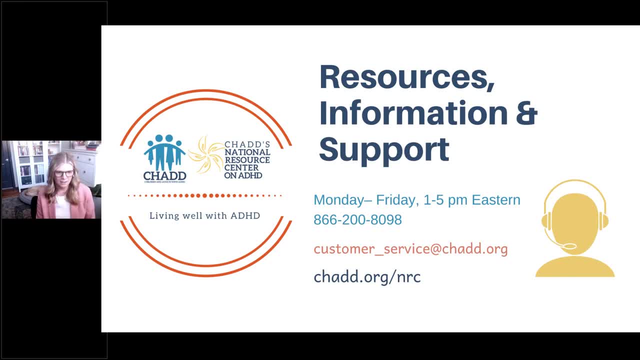 And gradually rewarding staying on task with their reading. You can also reinforce the like amount of pages that they read versus the time that they're spending reading, in order to reinforce a reward: actually getting through the chapter instead of how long it takes, And then they might. 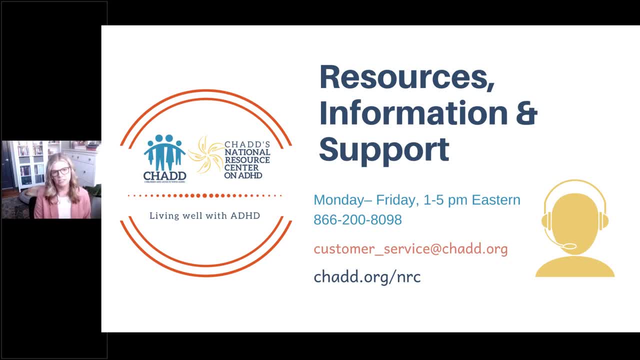 find that they're more efficient. Another thing that we've done in schools is finding kind of nonverbal ways to reward on task behavior And maybe you know if you're reading a book- you sometimes it's. you know if we have a jar and we're putting pom poms in a jar and each you know. 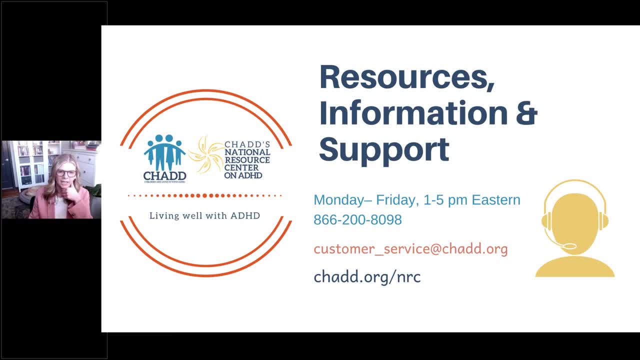 as a parent. you're just going to walk by while they're reading and monitor, And maybe you do it every five minutes, 10 minutes, maybe more frequent than that- And you drop a pom pom in the jar and it doesn't make a sound, So it's not going to distract them from the reading. But 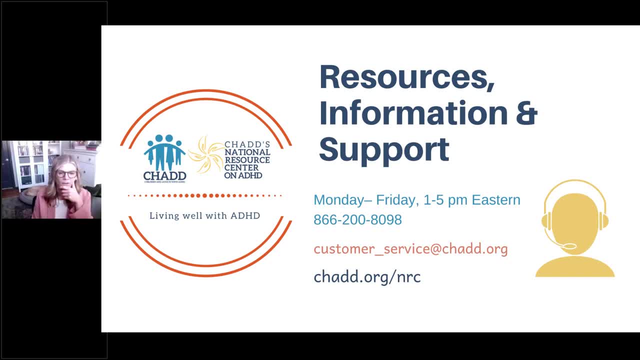 if they do happen to look up, they'll kind of see the jar getting fuller and fuller. So you're not stopping to praise them verbally, but you're reinforcing it. you know the time that's going by, that they're staying on task. Another idea is to sort of set goals around. 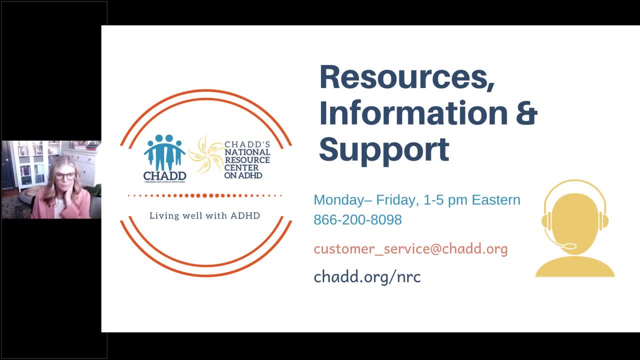 just getting started. Sometimes they'll get put off- put off chapter reading because it seems like it's going to require a lot of mental effort to get through. So you can kind of reward just getting started for five minutes. So those are some general strategies that I think work well. 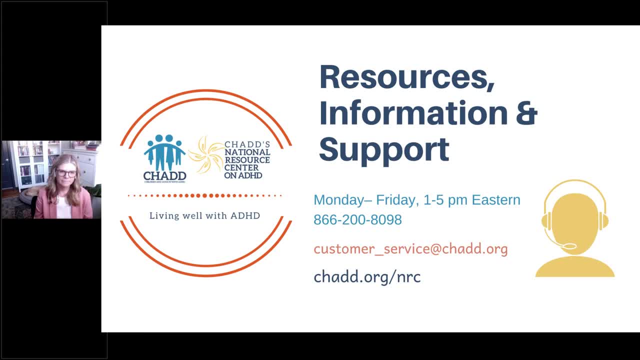 How does one align your program or the strategies and tips that you shared with the child's IEP, particularly due to probable frequent change? So the home program keeping in concert with the IEP. So sometimes we'll have specific organization goals written into an IEP, Sometimes they won't. 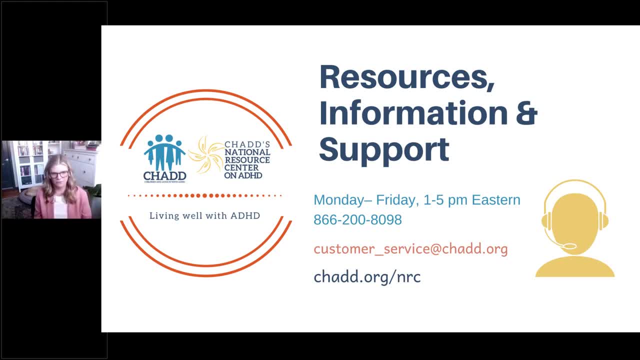 be because, you're right, we're gradually shaping these behaviors. the goals might change and kind of the way things that are worded and IEPs- they like them to be concrete and specific, the IEP goals, but they also- they don't change as frequently as you would need a point system. 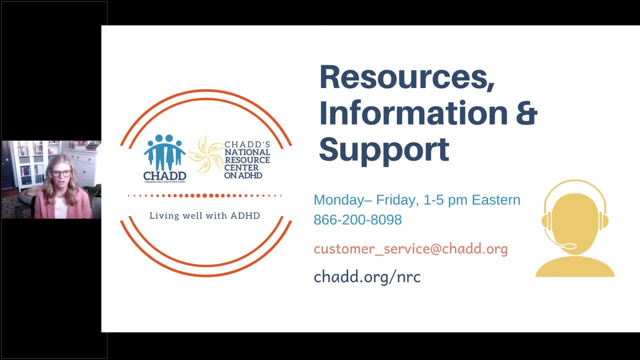 Yeah, Or checklists that you're using at home or at school to change as you're shaping behavior over time. Maybe they change once a year, sometimes even less frequent than that in the IEPs, So perhaps it can be written a little bit more broader or higher level of you know. 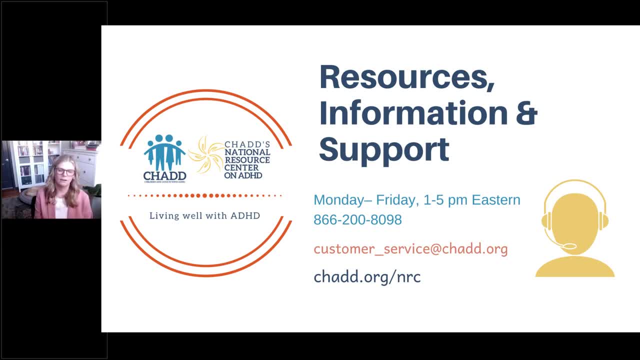 completing an organization checklist or working on homework recording with their, with their school counselor or their teacher. Another common like accommodation that parents ask about with IEPs or 504 plans is to have a checklist. I think one of our plans is reduced homework load for students with ADHD and whether that's appropriate for going in their IEP. 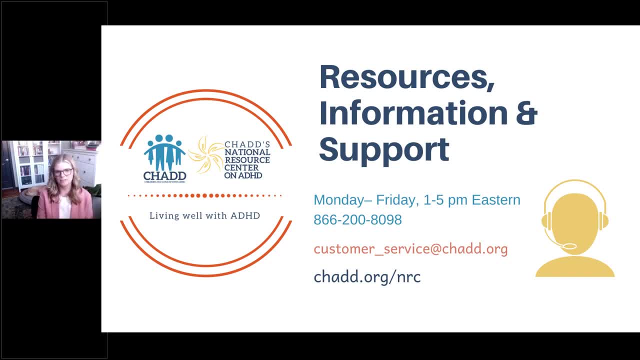 And that can be a double-edged sword. I think it's better if we focus on helping the student to build these skills So that way they have sort of the knowledge and the skills to execute these things even when those accommodations aren't in place. 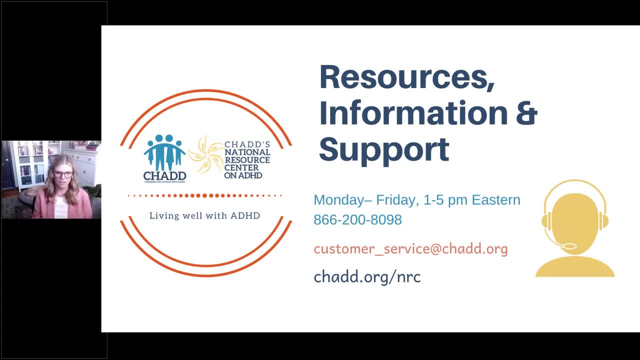 So we want them to be able to do the same amount of work as others Eventually, And if that's a goal, then it's not a bad idea perhaps to have reduced homework if they're not having any opportunity to even practice these homework and organization skills. 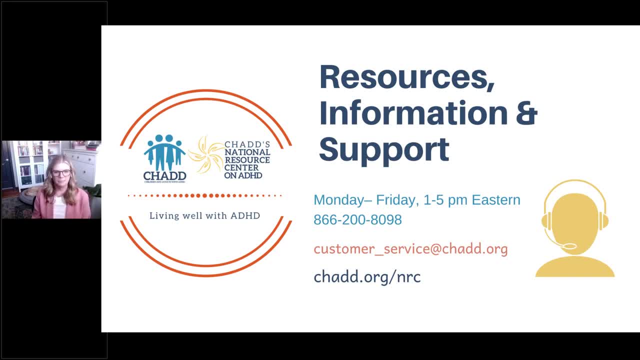 There's just no time amongst everything else, but that could be done more temporarily. So those are some different ideas for for considerations with IEPs. I really like the planning aspect, but I'm a little indecisive about using the reward system. 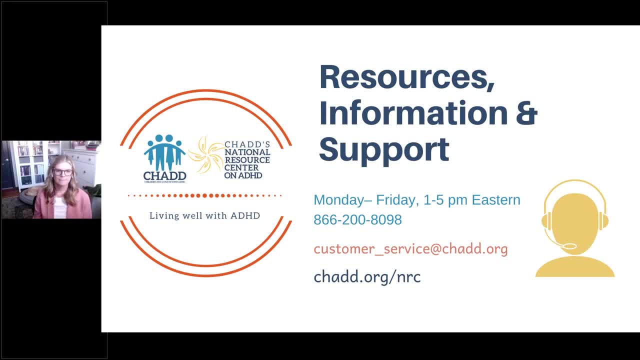 Is there an alternative, as this parent would rather her child notice the positive outcomes instead of expecting something in return For starters, you know how is that working right now? If that's something that is already, it's natural, so it's already been in place, and 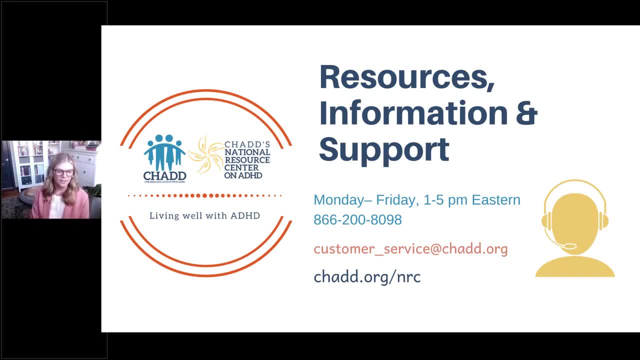 it's shown that that's not motivating in and of itself, then that's: the goal of this work is really to get them going on practicing the skill of planning ahead. So that way it is that it is motivating and just sort of understanding how executive. 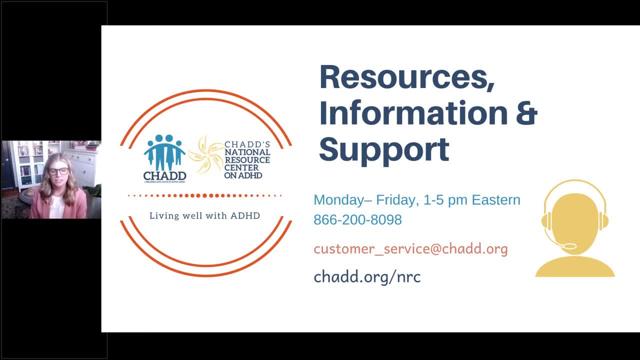 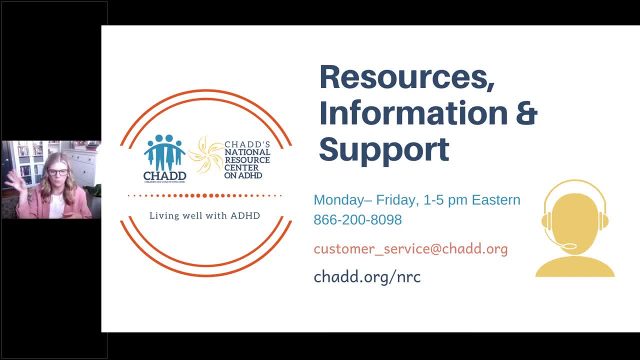 the short term is that we're sort of breaking down those longer term goals to make them more short term. And rewards, You know, can also be. they can look different for different families, They can be privileges, They could be things that you might do anyway, but now you're just structuring when you do them. So you know. 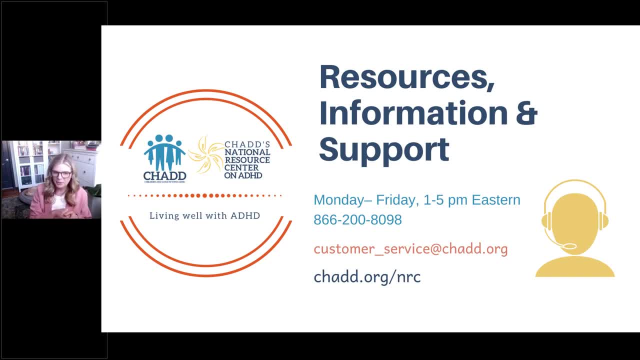 once you come home and you've completed your homework or you've written X amount of tests and projects in your planner, then you will have free time. So you can sort of set it up as like a win then just structuring their day after school and how they use their time And that. 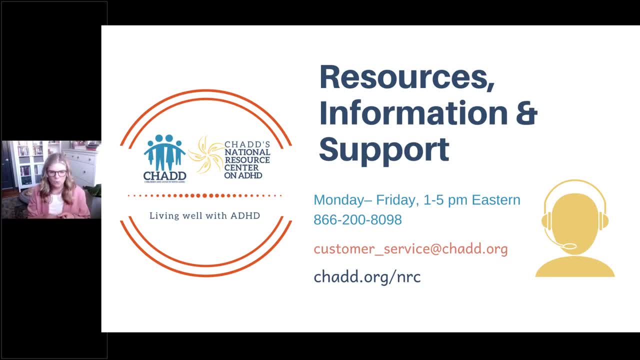 can kind of be their own privilege. It's not necessarily like a reward that you have to go out and buy something for, but just sort of structures around something. maybe they would have earned anyways. but you're giving it to them for doing a certain behavior And that's. 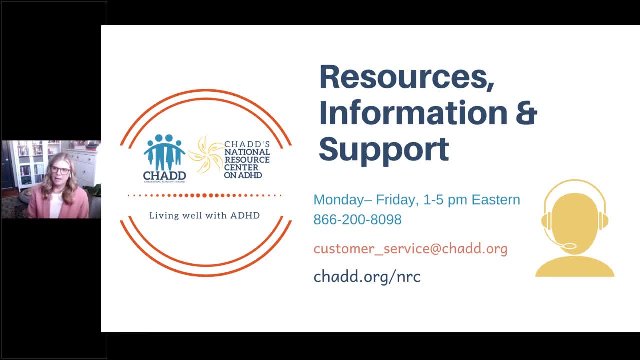 something that can happen daily. What we also see is that they experience this external reward being given to them helps them to just even try the planning skill. That's what we're trying to get them to do: Try it out and get better at it over time And so. 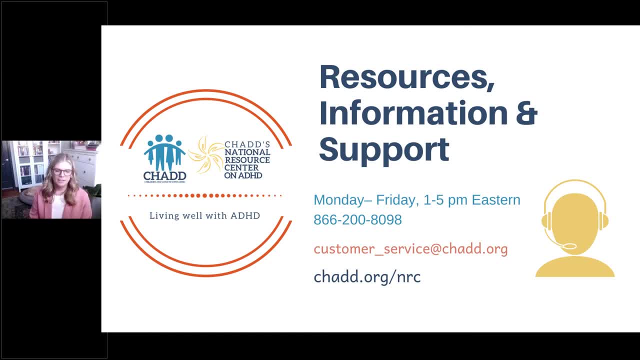 if we're able to motivate them to try something this way and then they're successful with that, that success that they experience will be an internal motivation And over time that will be enough for some to drive them to kind of keep doing it on their own without another reward. 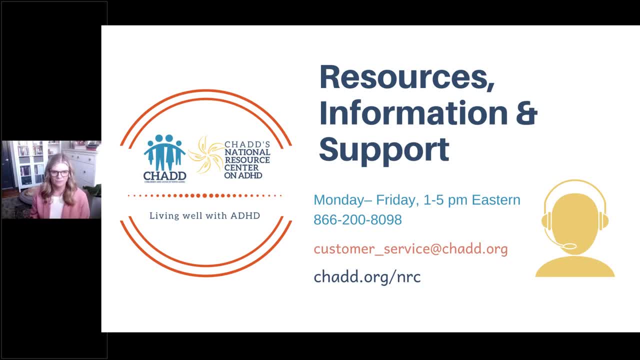 but working towards sort of that end, all goal that everyone agrees on- of better grades and school performance. We know that there are many parents with ADHD who also have children with ADHD. Do you have any suggestions For these parents in terms of not taking over their child's projects and their homework, etc. 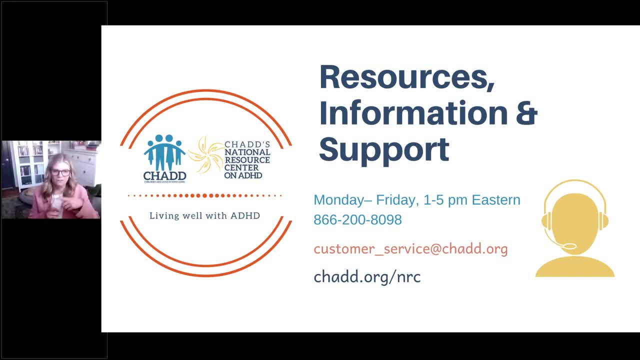 And I would say it comes back to kind of setting up goals that are feasible and that you can do consistently. So for the parents: if you're a parent with ADHD, set up goals around checking their planner and their calendar to see that they've been doing these behaviors in advance. 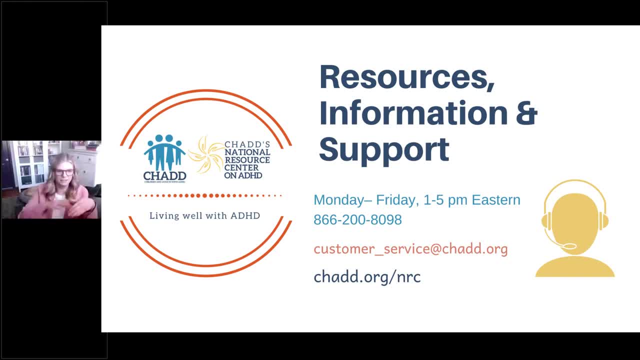 before something is due, that they know what the project sort of subtests are to be completed and that they've kind of assigned times to do them well before when it's actually due. So that way you've got the smaller chunks done in advance And set up a system that works. 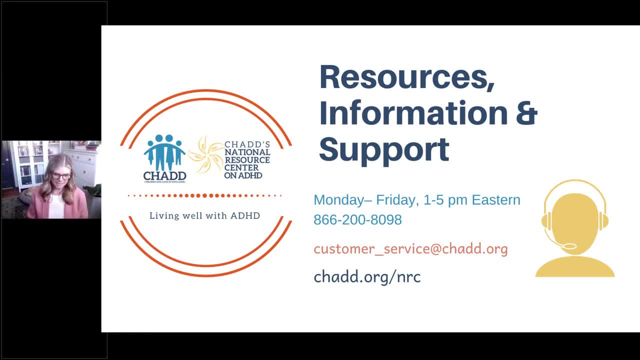 for your family. that's feasible for your family to do And it's something that you can kind of do consistently, because number one thing with these systems is making sure that you're able to consistently check and consistently give rewards, And if you have sort of different, you know. 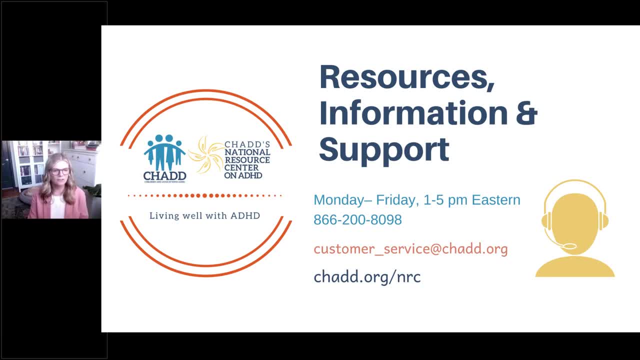 work demands, life demands, parenting other children being difficult especially, and then compound that with having your own ADHD sort of stay on top of all of that And so setting up a system that's going to work for you and your family, that you can do and implement or use. 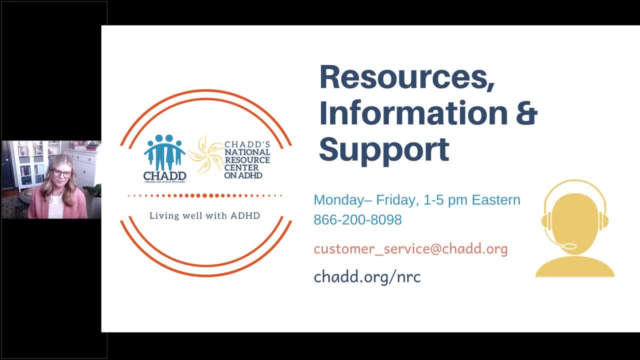 consistently, You know. and then some of these strategies that we're talking about, of using a planner, setting, you know, an alarm or reminder for yourself. those are strategies that the same sort of organizational time management strategies that we use with our emerging adult and college. 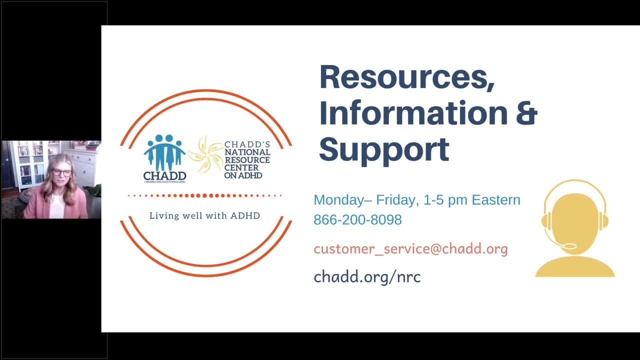 populations, and they're useful for adults too. So these are strategies that you can also, as a parent, use for yourself and sort of set up your own structure, your own system for getting tasks done and having sort of checking and monitoring their homework and their project task completion. 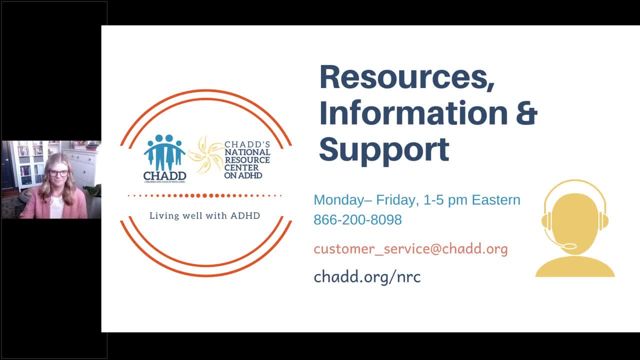 in advance as well. I would like to thank Melissa again for a wonderful presentation and our participants for taking time to join us today.